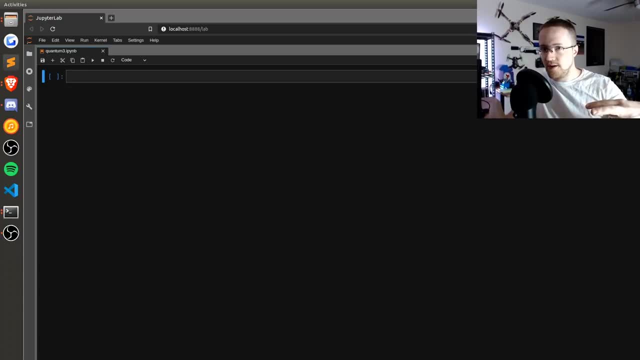 In terms of how many, like, say, cycles through the circuit are required to get the answer, But also the reason. it's more so. it's not just the speed, it's why is it faster? So this is the first time you should get a real idea and feeling for how is this working. and then, why is this working? because the reason why it works is the circuit is able to consider all of the possible inputs that could have come into the circuit, and it can. 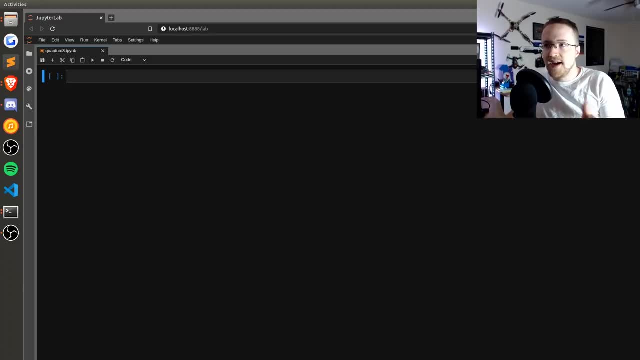 immediately respond with the, with the output. So, and the output is not output based on input, It's output based on the nature of the circuit. And so that's what's cool about this algorithm: It's not the, it's not the actual result of the algorithm, And I think that point gets lost on a lot of people. I at least, when I'm looking around at explanations and stuff of the Deutsch-Yosa algorithm, as well as some of the others, like the Bernstein-Vazirani and even Shor's algorithm, although we, I think, most people- 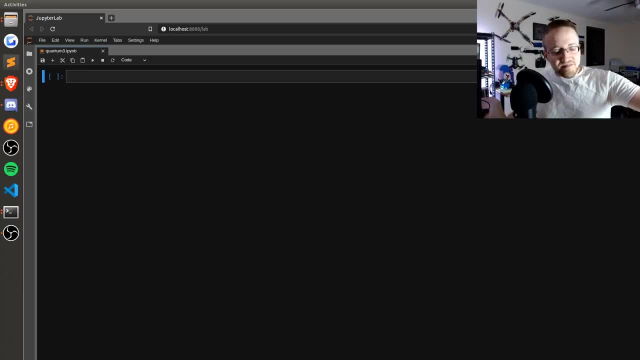 understand. Oh, it breaks encryption, Cool, OK, But the Deutsch-Yosa algorithm is the inspiration behind Bernstein-Vazirani, Shor's algorithm and I'm sure many others, because it shows- and this was kind of the first one that shows: oh, you could do this stuff like this. These are things that you just can't do with a regular classical circuit. So let me just formulate really quickly. I don't want to spend too much time explaining the problem, but it would probably 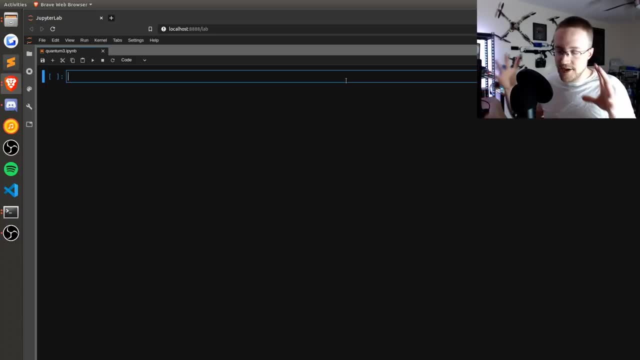 be a problem, be useful to explain the problem. so with the, the Deutsch Yosa algorithm, you've got a function right. so the function is your black box and let's say you're gonna pass a two-bit string to this box and the. the question that we want to answer is: is this black box going to output a constant output? 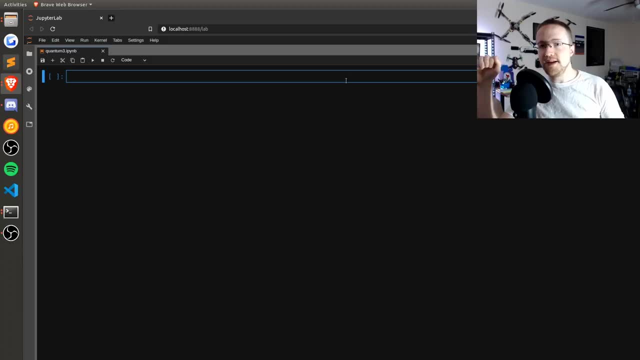 or will the output be a balanced output? so will this box always output all zeros or all ones, or will it output zeros and ones in a balanced manner, so an even number of zeros and ones? so with the classical circuit, the only way that you could find this out is it is that minimum. 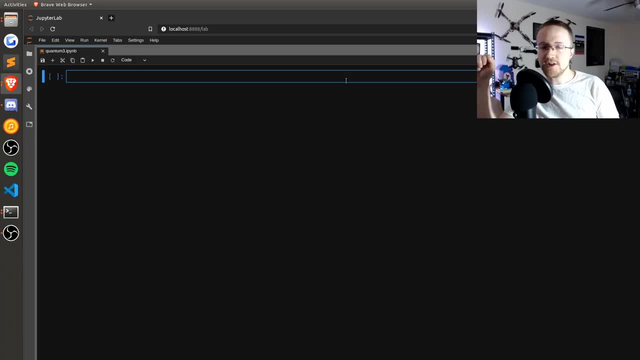 two, you would need two outputs from the machine. so if we got a two-bit string, it's going to take at least two queries, because on the second query you could find that, oh, there's a, let's say, on the first query the result is a zero, zero. the second query: you got a zero one right, so that's going to. 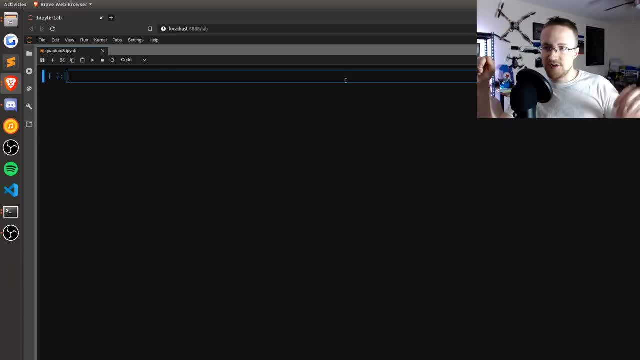 do that right. and when I say query I mean like pass through the circuit. so to find out if a circuit is balanced or constant on a two-bit string, it's going to take at least two passes as we increase the number of bits in the string that we want to pass through this function. 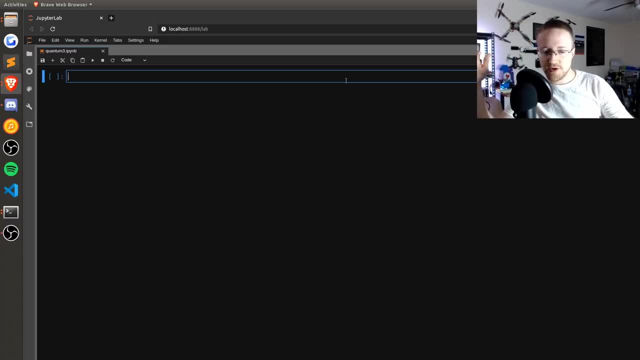 it's going to take longer and longer and longer for a classical circuit to be able to make this determination. a quantum circuit, on the other hand, can make this determination regardless of how long the two-bit string is in one pass. and this is what shows the power of quantum circuits. and again, the 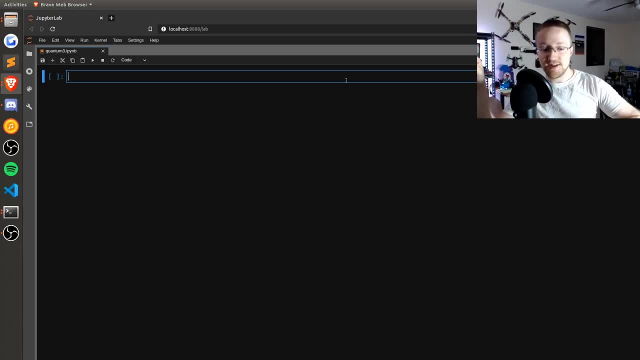 the problem itself is not useful. it's just. this is the most basic representation that we can come up with that shows the attribute that quantum circuits have that classic circuits do not have. so don't get hung up on the problem, um, get hung up on why this solves this problem. So with that out of the way, let's go ahead and get into it. 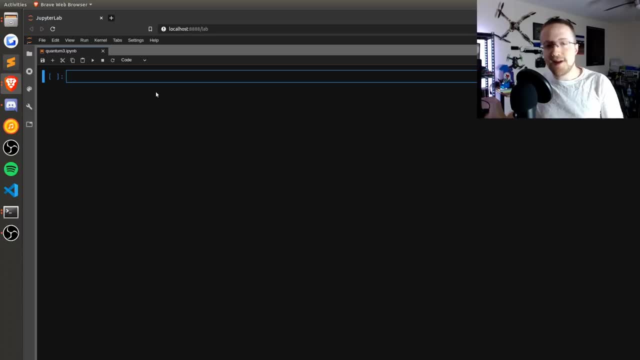 So, to begin, this all rests on a term that I'm going to coin as Hadamard sandwiches. So again, like I said in part one, I'm not a quantum physics expert. okay, I'm not even a physics expert. I'm really not an expert of anything. So remember, you're just watching. 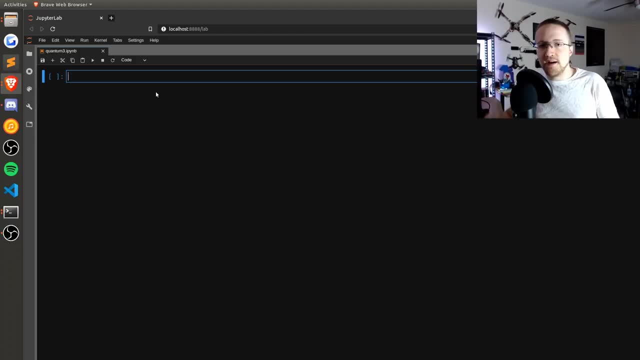 a dude on YouTube, So I'm going to use words here that I feel describe what's going on, but they're probably the wrong word. So, yeah, just bear with me there. If you're like an actual- you know, PhD person, feel free to correct me and tell me that the word is correct. And if I've 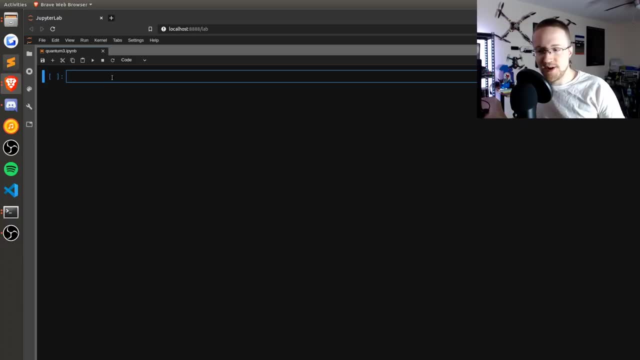 somehow stolen Hadamard sandwiches. I apologize, I'm pretty confident. I've never seen that anywhere. but that's what it looks like. It's just Hadamards on all the sides, So you're just squishing something between Hadamards. It's a Hadamard sandwich. So anyway, if there's an. 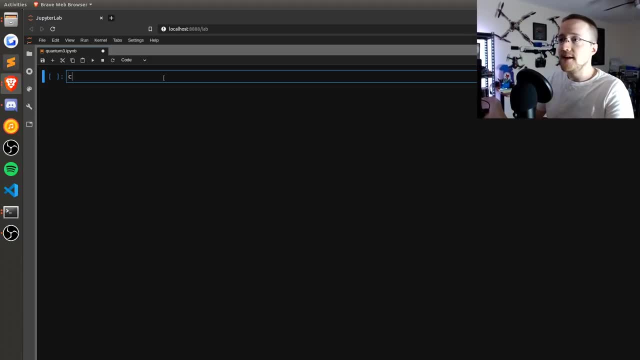 official term for it. let me know So to begin. well, we're probably going to need some of our initial imports. huh, I don't really want to type this out. Everyone should have these. so I'm not going to do that again. It's a waste of time. So we will have a kiss kit. I did check. 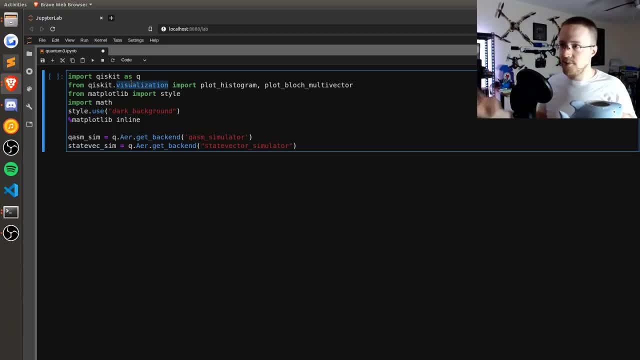 this, by the way. By the time, this video is coming out after part two, and I'm sure people will, but I don't know which one is the new one, but this happens all the time in libraries. I'm going to go with the shorter one, but you can import both of these from the shorter one, So cool. 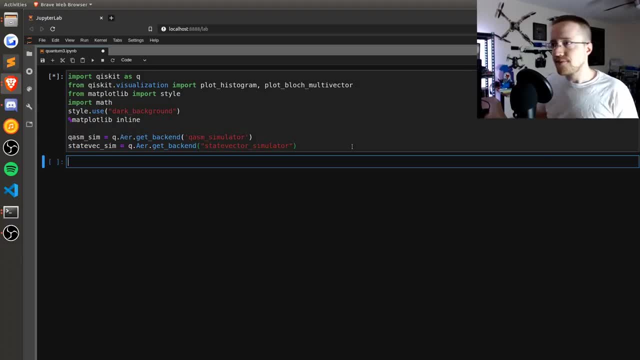 So yeah, all this stuff is stuff you've seen. So the first thing I want to do is show you this Hadamard sandwich on what I'm also going to call uncertain qubits. And when I say an uncertain qubit, this is a qubit that will collapse. So I'm going to call it an uncertain qubit. 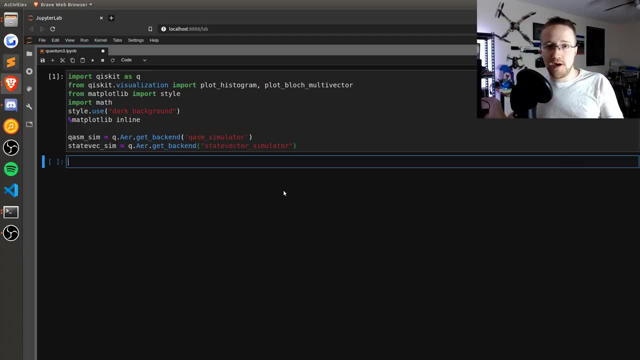 So, to begin, let's say we've got a circuit and that's going to be a quantum circuit, and we'll give it, we'll make it a two and two, So two qubits, two classical bits, And then we'll say: 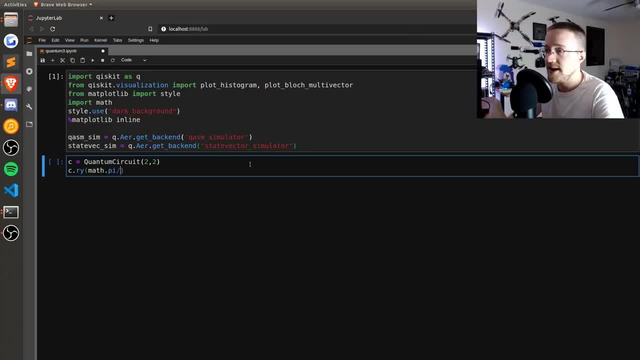 rotation on the y and we'll go with mathpi divided by four on qubit zero, And then we're just going to do the same thing to qubit at index one. So that's, our two qubits are done, And then what we're going to say is: I'm going to call this a ridge state vec and that's going to. 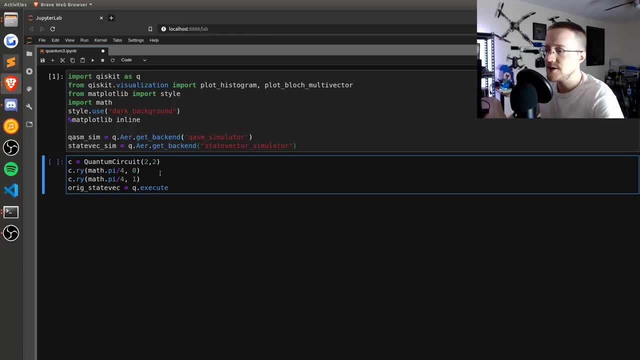 be equal to qexecute And we're going to execute the circuit on the back end of this state vec simulator. So just remember you need, if you want to get the state vectors, you have to do it before you actually take the measurement, Otherwise the circuit will have collapsed. 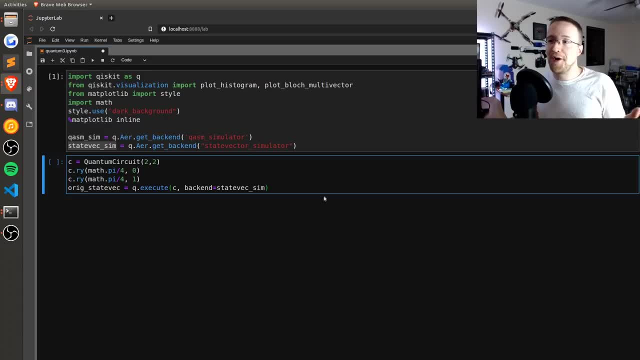 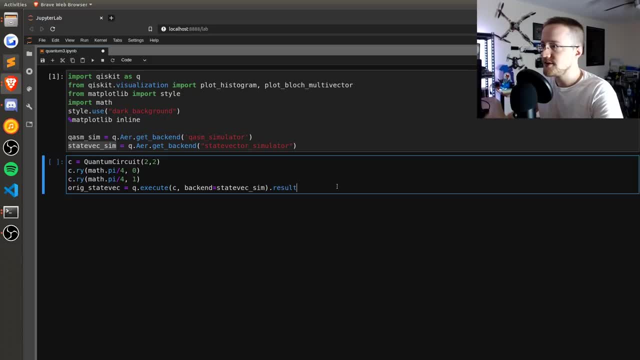 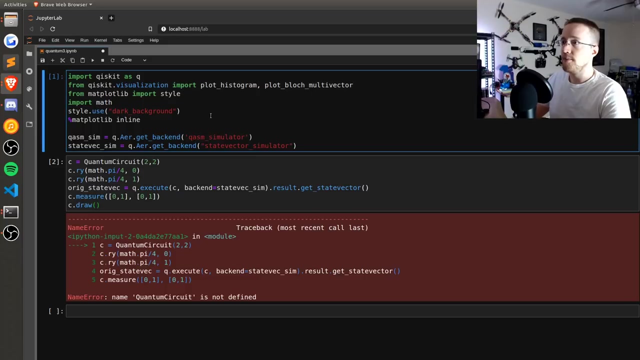 state vector won't work, So state vec, sim. And then we're going to say, dot result, dot get state vector. So now we have the actual state vec And then we will c? dot measure, And then we're just going to measure both qubits to both classical bits, And then we'll do a c? dot draw. Oh, 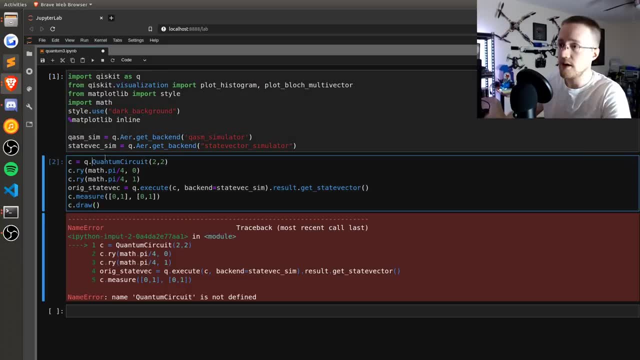 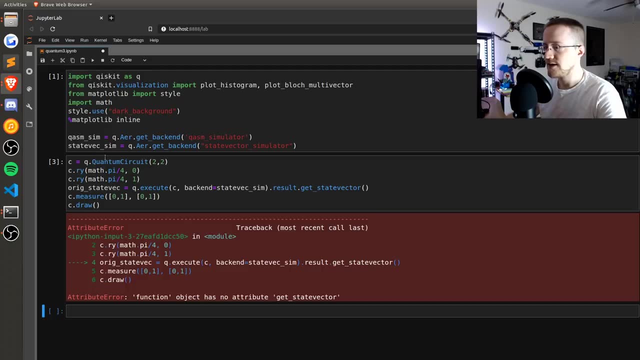 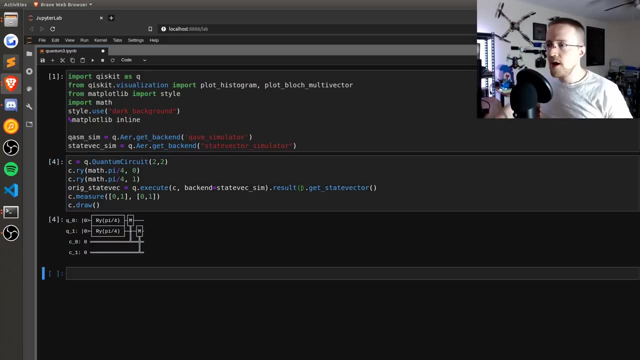 q dot quantum circuit. I see q dot quantum circuit. I screw it. Hopefully I didn't get anything else up. Get state vector. Why not Results? Oh, we didn't call result. It's early in the morning, Coffee's still setting in. Cool, Okay, So we have. 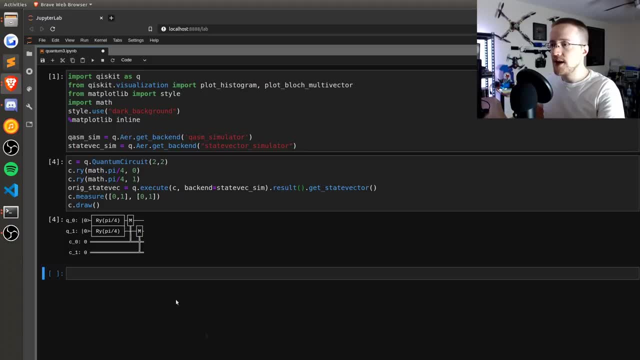 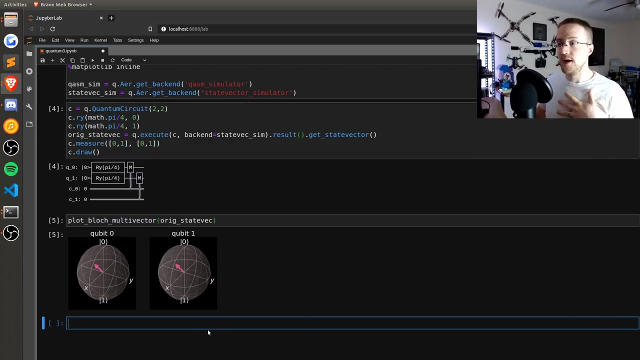 our rotation, our measurements Great. So the first thing I would want to do is let's plot block multi vector And then we will do the original state vec Cool Run that All right. So that's how the original state vector appears to us, before we've done anything for any Hadamards or 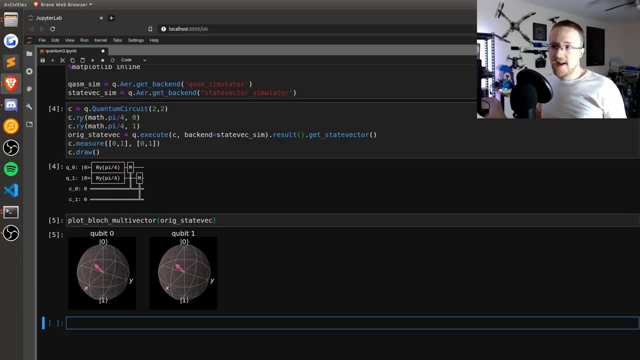 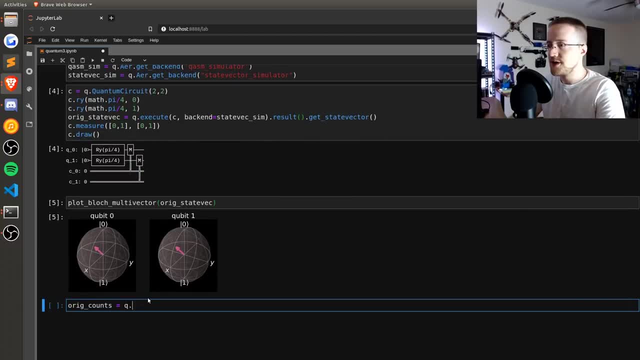 do a couple rotations on the Y, And then we're going to do a couple rotations on the Y, And now let's do a ridge counts equals Q, dot execute And we will execute that circuit. We're going to say back end. back end equals the chasm underscore. sim shots will be 1024.. I'm going to make this pep. 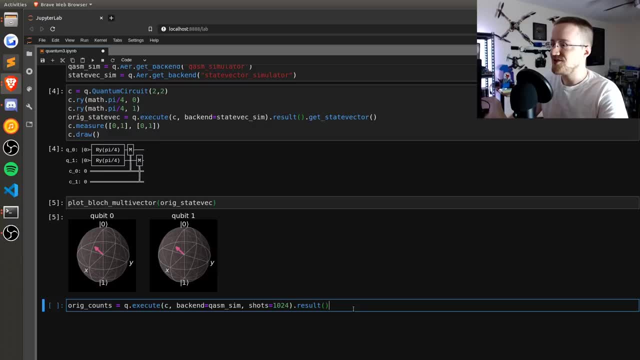 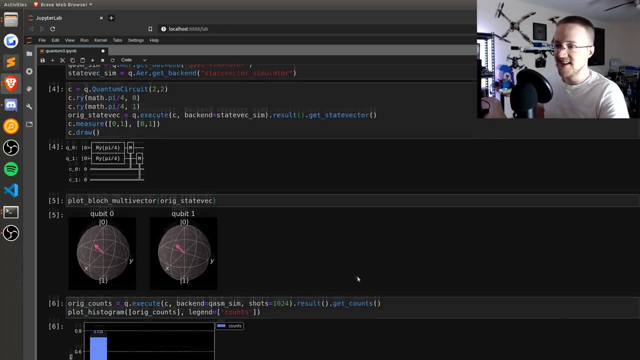 eight, And then we will do dot results, dot, get underscore counts, And then we will plot histogram or ridge, ridge, underscore counts, And then legend equals. probably don't even need a legend here, honestly, but I'll put it in. So this is our distribution, So it's going to be important. 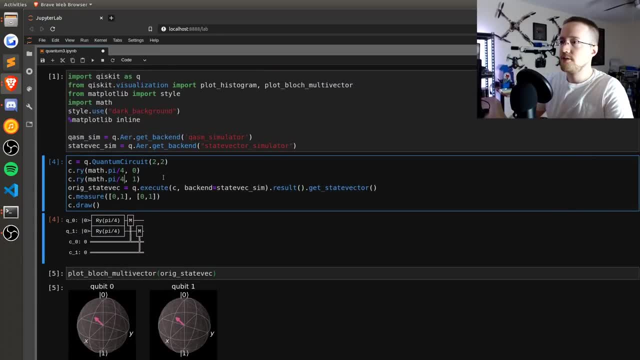 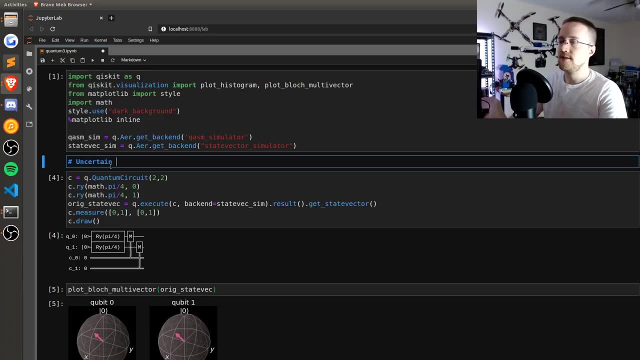 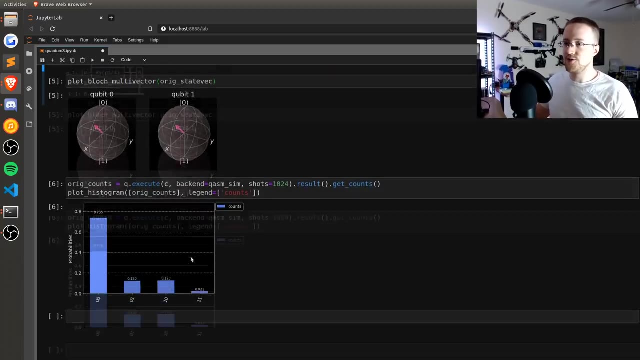 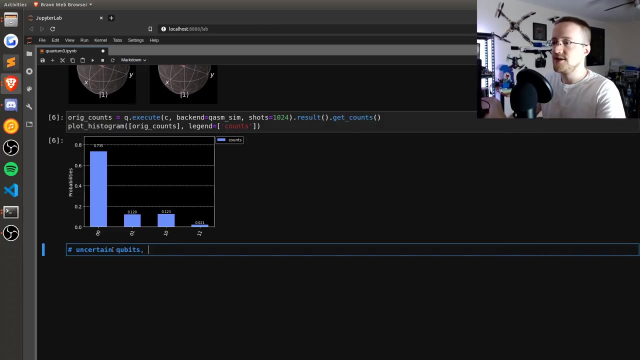 because first we're going to whoops trying to get an above here. First what we want to do is uncertain qubits. let's say So, this is for uncertain qubits, just naturally, this is what they look like. Now what we're going to do is we're going to do uncertain qubits Hadamards at. 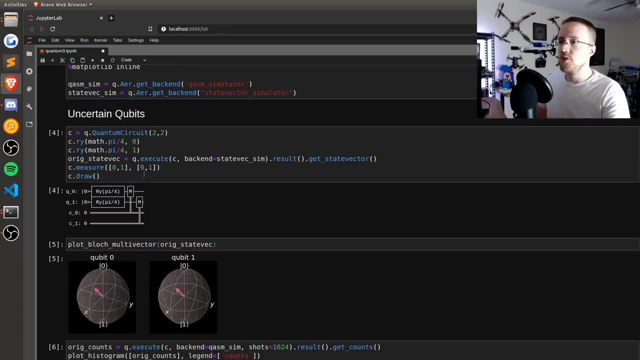 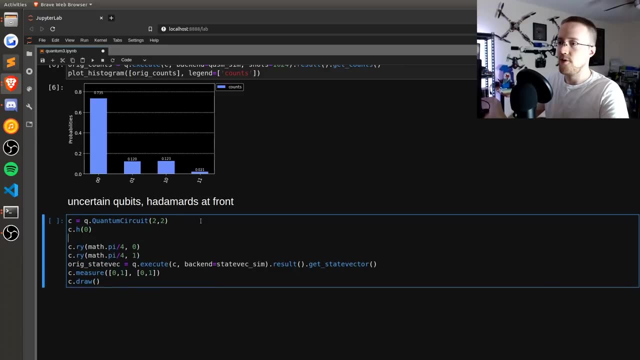 front. Okay, So all we're going to do is we're going to take this copy paste and now we're going to do the same thing we did at the beginning. So, Hadamard on zero, Hadamard on one, That's our. 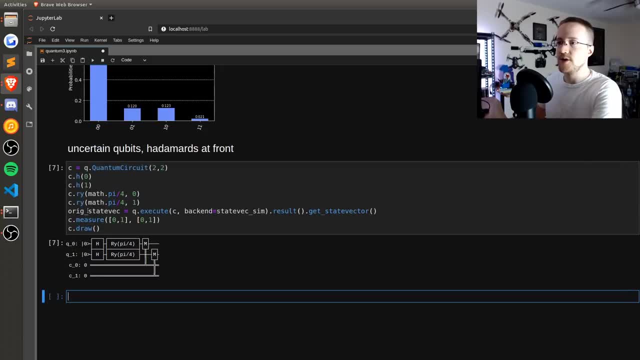 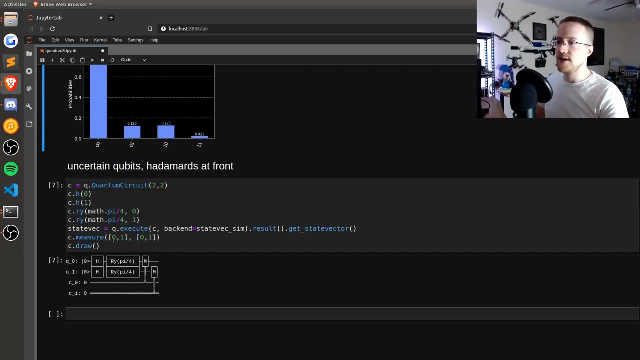 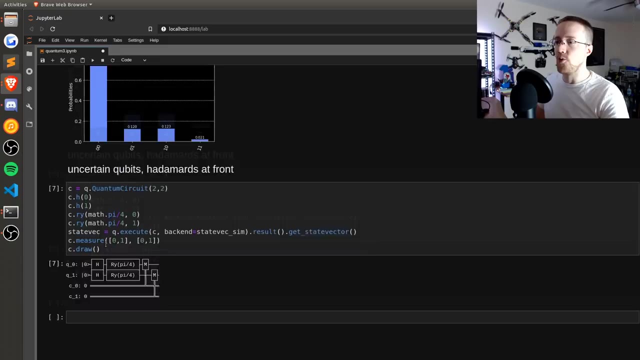 circuit. Cool. We don't actually want to say ridge state vector, That should be reserved for the original, And then we're going to do the counts as well. So we've got a state vec draw. I guess we'll- we'll first, we'll do, we'll do everything in the same order. I don't want to make it. 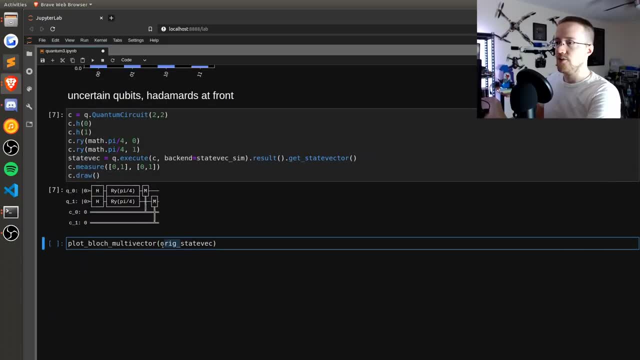 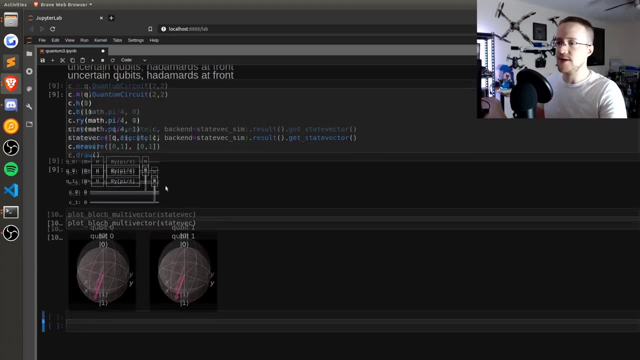 confusing as I'm scrolling through here: A ridge, state, vec or actually state. do we not run? No, we did run this. I think I just ran it before I made the change. So, as you can see, the the single Hadamard actually made kind of a significant difference. 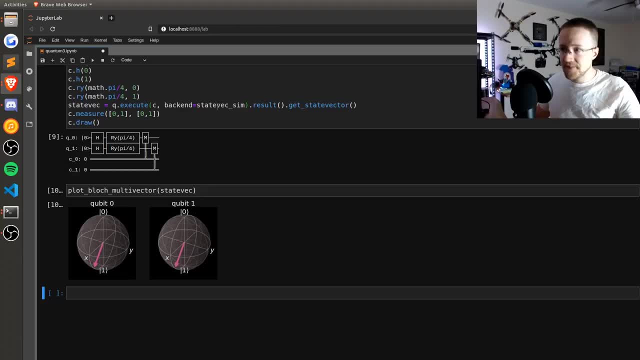 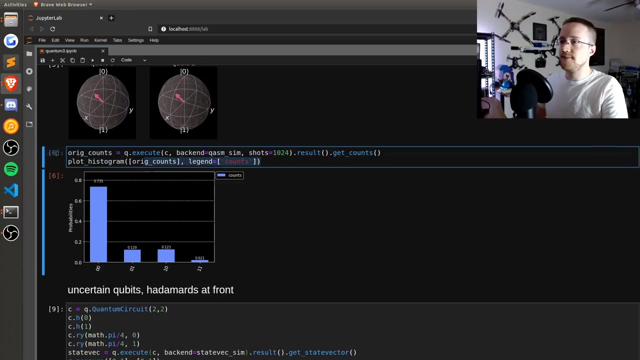 right. So there's that. And then let's go ahead and plot So like: okay, that's how it impacted the actual block multi-vector, but how does it impact the actual distribution? So let's do this: How do these actually collapse? What would it actually end up? 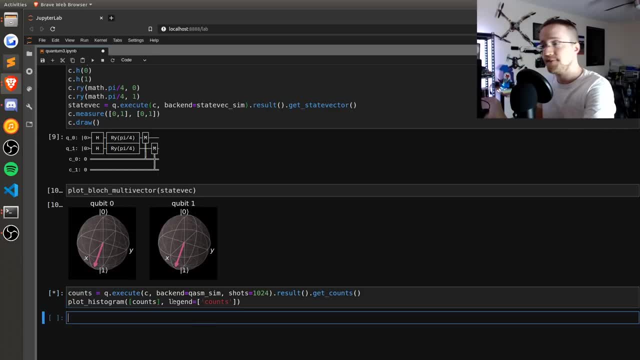 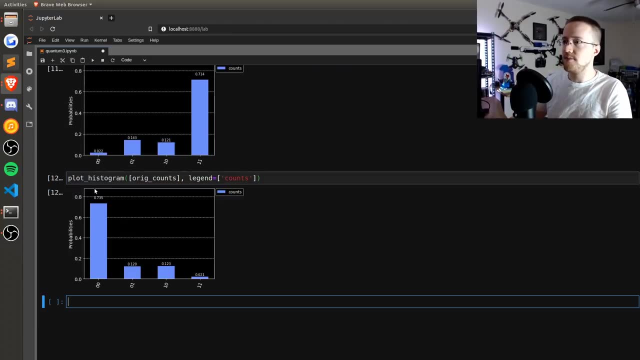 Looking like so counts, and then I'll just paste counts. So if we look at this- and in fact, let me just just to make it easy, I'll get rid of this after we're done- But so this was the original. it looks as though probably 01 and 10 are unchanged, But really, what happened? 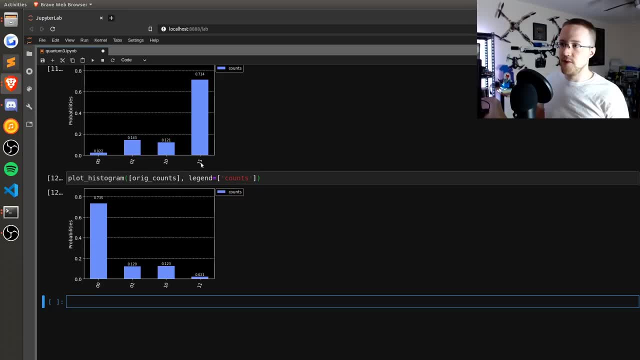 is everything just flipped right. So now 00 is as frequent as one one was. these are stay the same, cause they'd flipped, And then one one, you know, flipped them. so why wouldn't they do that back? Yeah, I'm sorry. All right, So grids are then on the same order as the original and the same order. But that's G'vec, just—. And then the one Yes, And then let's go on. Dootf, say um data journey on the 2C, Because our- And initially we're- WillyRY- I was� who we do- We 3 dustin left the tree. We didn't pay attention to X спис. 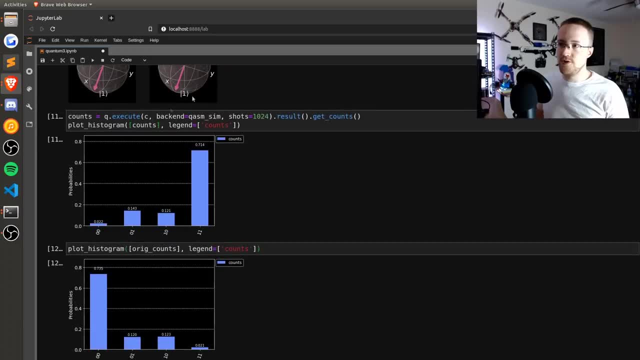 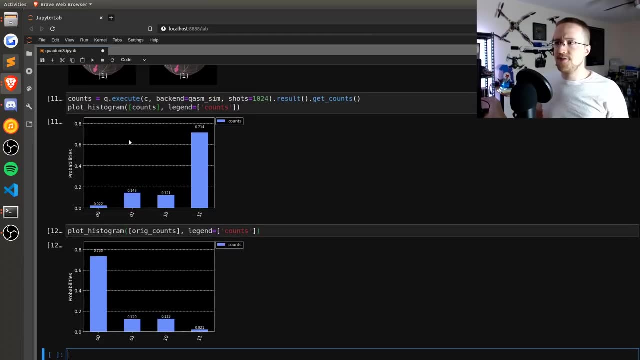 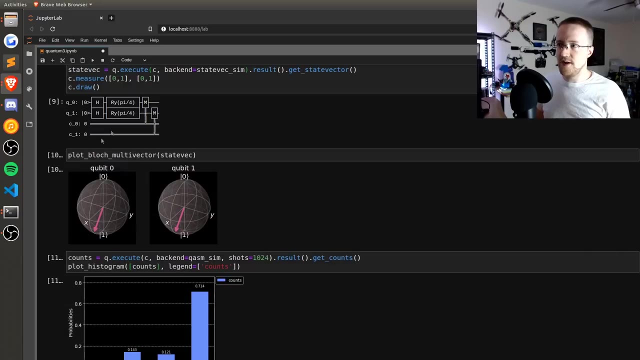 it, you know, flipped basically with zero, zero from the original. so applying the hadamard did something kind of funky here, because instead of um, you know they were already uncertain. so then you applied the hadamard and then it. it flips them around right and also changed that multi-vector. 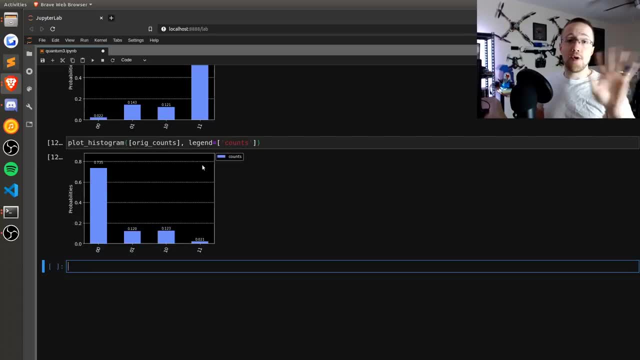 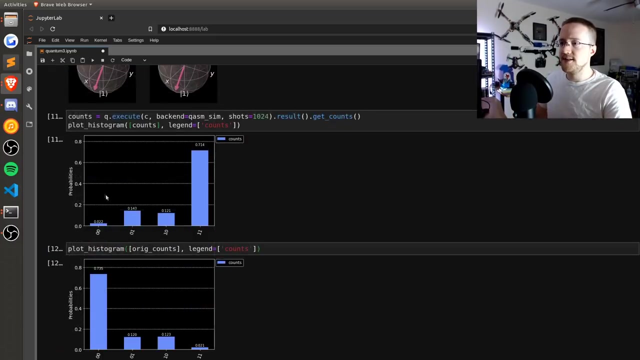 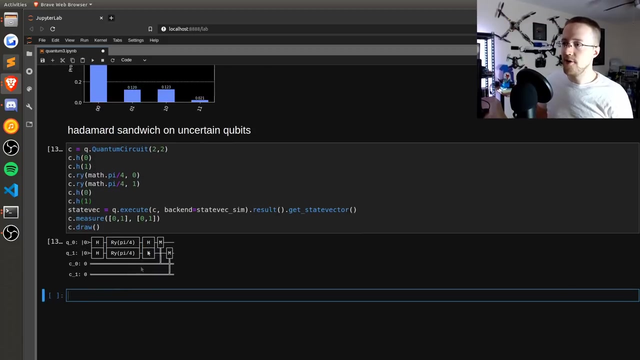 pretty significantly. but that's a hadamard in front. now what about the um, let's say, a hadamard sandwich on uncertain qubits? um, and all we're going to do is take this paste and now we're just going to wrap hadamards on the other side. so now you can see hadamard, hadamard, hadamard. 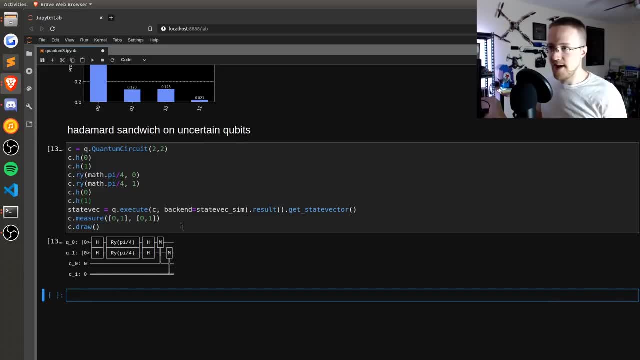 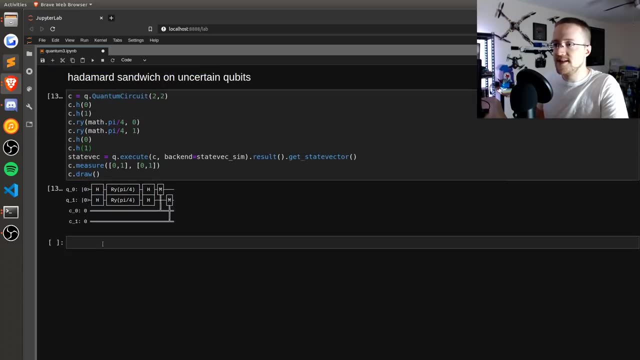 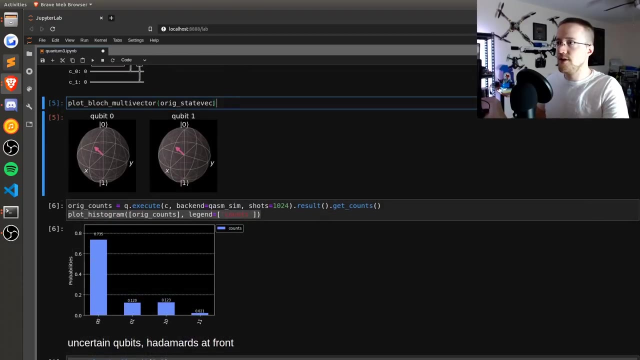 hadamard. so it's just squishing in these qubits around hadamard gates, hence the hadamard sandwich. uh, so now let's take this, let's look at the state vector that this produces, and, um, um, let's go back up to the original, just because i think scrolling around is kind of confusing. 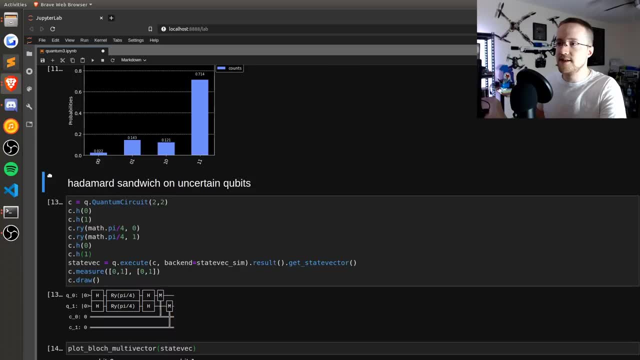 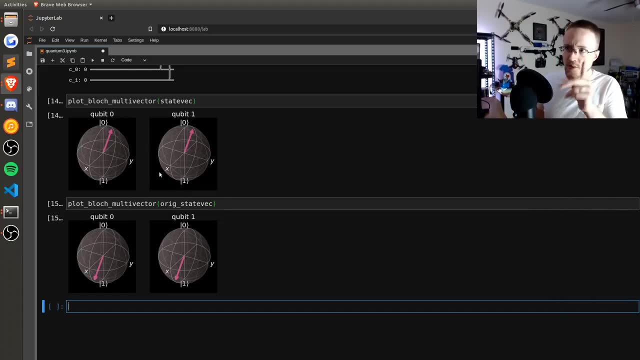 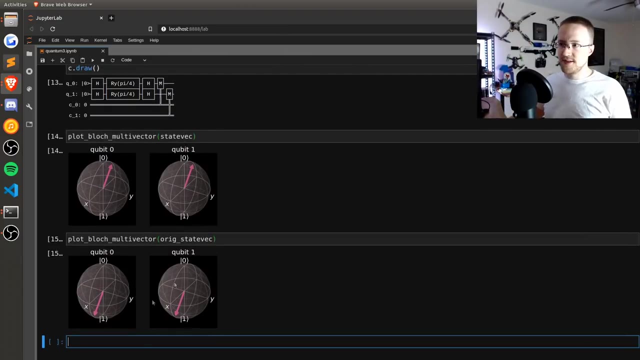 uh, and in fact i'm going to. i'm just going to delete this because i don't want to look at it. um, and come down here. i just want that to be confusing. now, when we look at these, isn't that interesting. so this is the hadamard sandwich. this is your original. no hadamards. now this is on again. 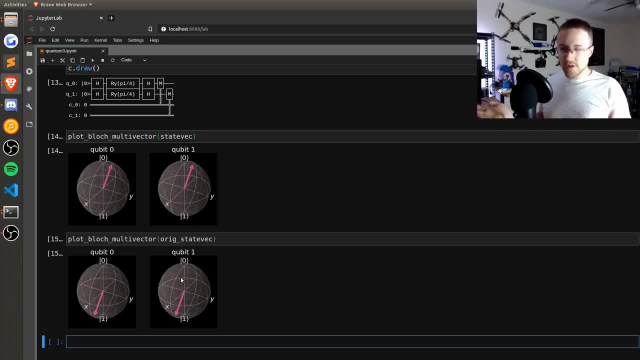 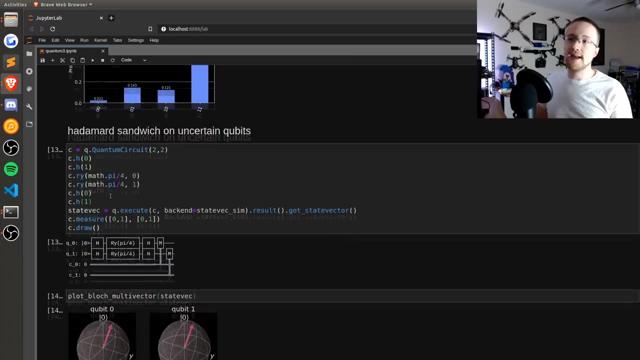 uncertain qubits that starts to look like: wow, it's almost the same. it's just kind of flipped right, but doesn't it look like if you were to guess where these are going to collapse, would you not guess that? like, if i was to guess, i would have guessed that this whole like flipped 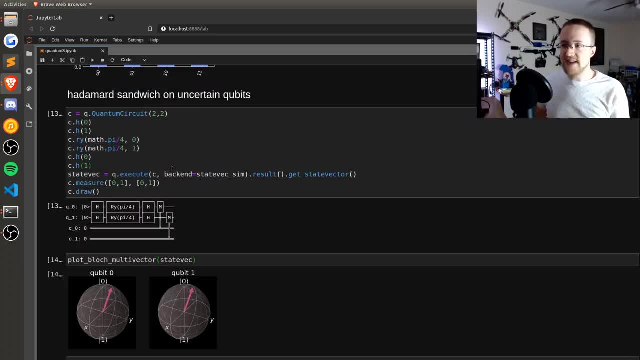 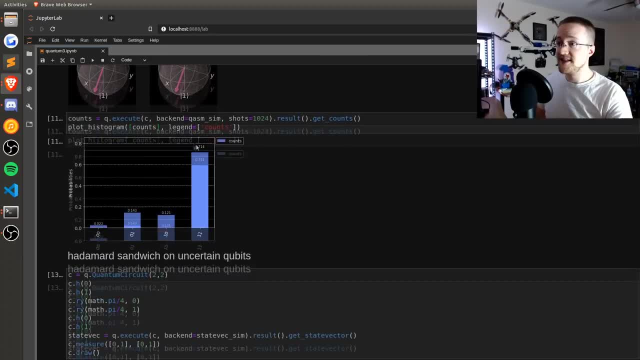 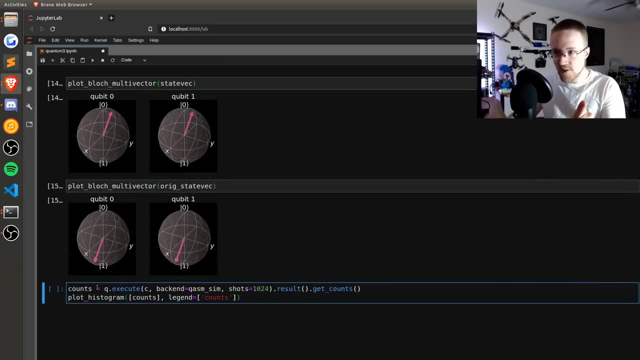 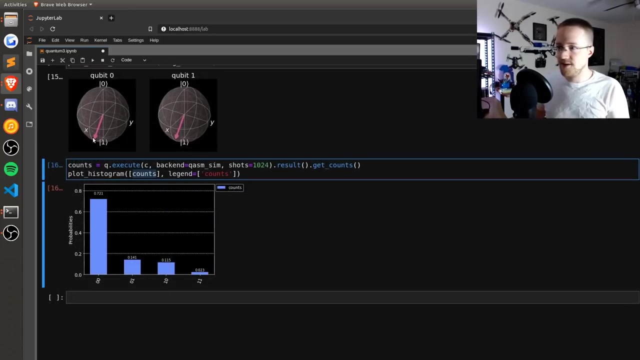 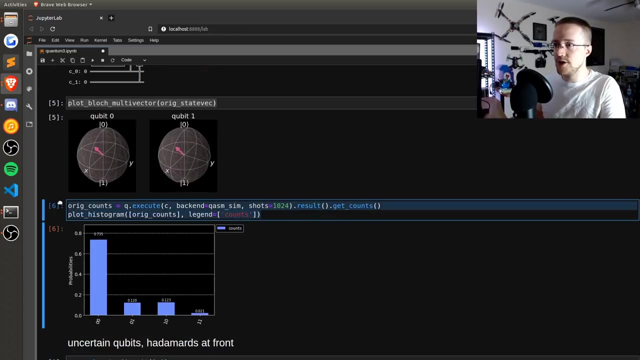 so i would expect that kind of flip there, uh, but instead spoiler, spoiler alert. uh, here's the hadamard sandwich distribution: right counts, regular counts, just the circuit we just ran. that's what that looks like. now let's go up to our original distribution. i'm just going to copy it. 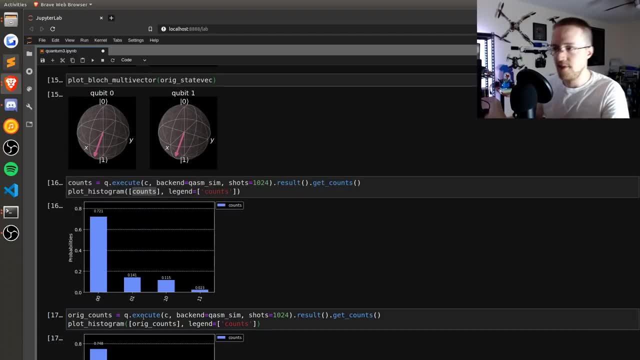 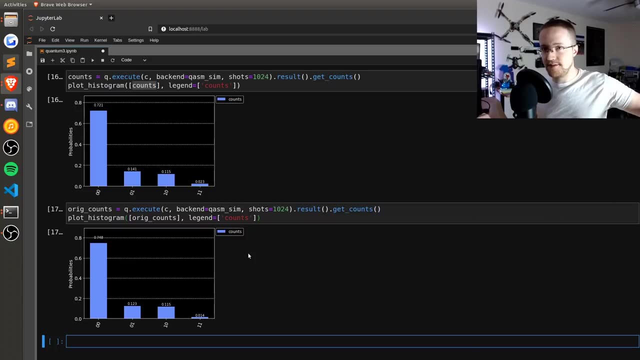 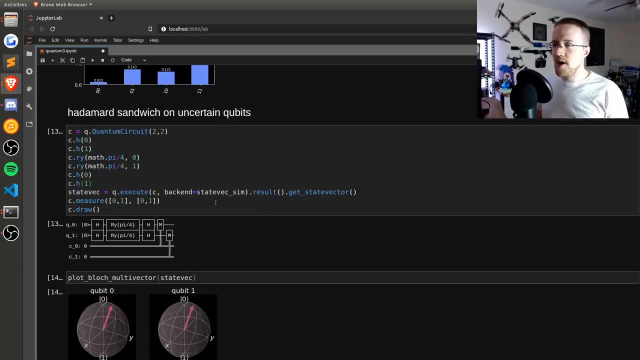 scroll down here: hadamard sandwich on top, original on bottom. it turns out they're the same. they give us the exact same output on the distribution. but so what happened though? what happened for us is, even though the output is the same, so the circuit output's the same, what? what we got was the possibility to 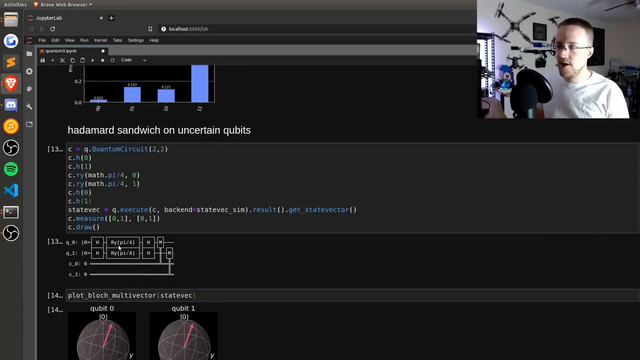 like at this point with these qubits here. we could have done something interesting at this stage in the circuit. we could have had another qubit that does something else that works off of this state here before we get to the final head of mards and then take our measurements. 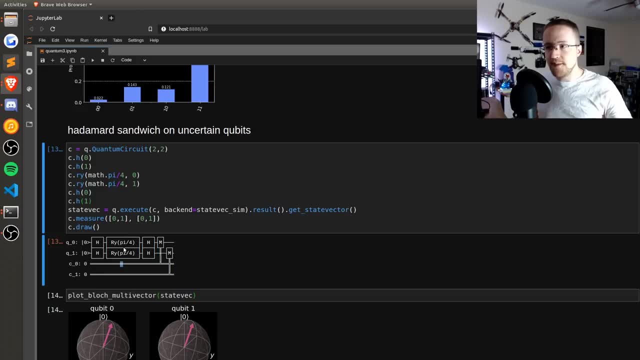 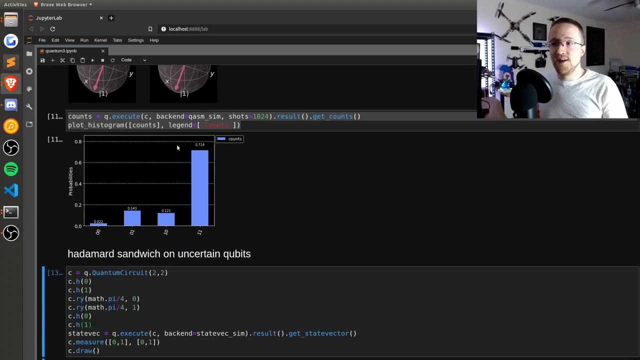 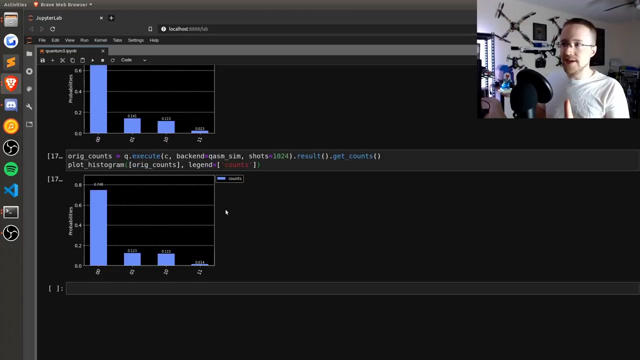 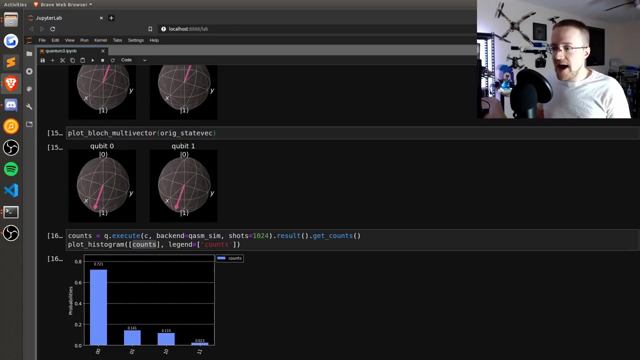 so so if we add one more qubit, we can do some something based on this superposition state, that is, basically querying all of the possibilities of input into the circuit without impacting the actual output, which is very interesting. so so that's with an uncertain, uh, uncertain, qubits. the next question is: how does this look in front of certain qubits? so imagine: 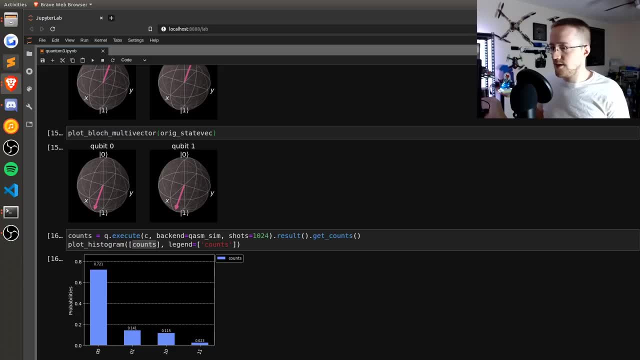 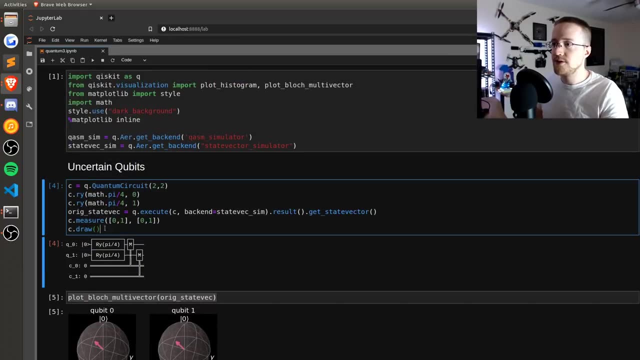 um, let's go with. i guess we just do the same thing and then we'll do maybe a knot or something. so that was uncertain qubits. so let's just come down here and let's say certain qubits, and just for the record, all of this, 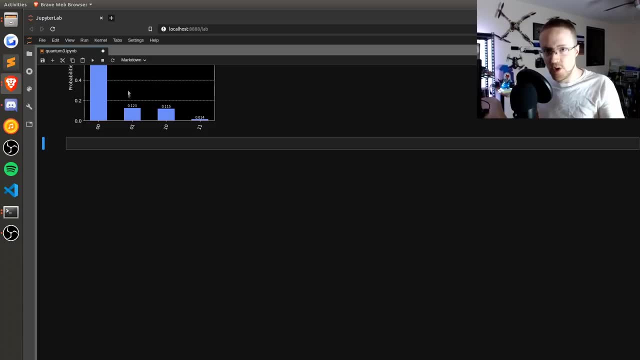 that i'm showing is completely applicable to the deutsche algorithm, as well as all of the other fancy ones that everyone's ever heard of it's. this is the concept that is uh important, so i'm not just wasting your time, i promise so. uh, now let's look at hadamard. uh, let's look at certain qubits. 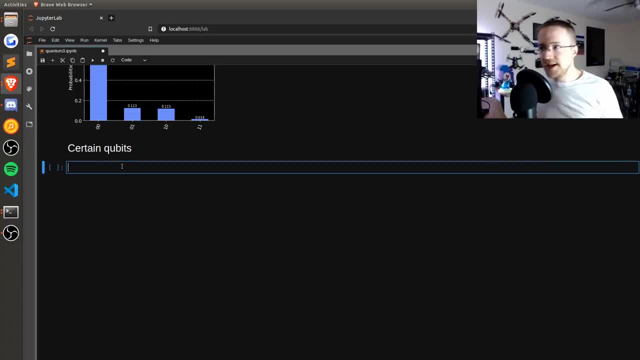 again. i don't know if that's the right word. i just that's. that's what i'm thinking of when i look at these, i'm like, okay, this is always going to collapse in such such a way. so rotation on y is uncertain, but we could either do nothing or just to do something. let's just do a not gate. 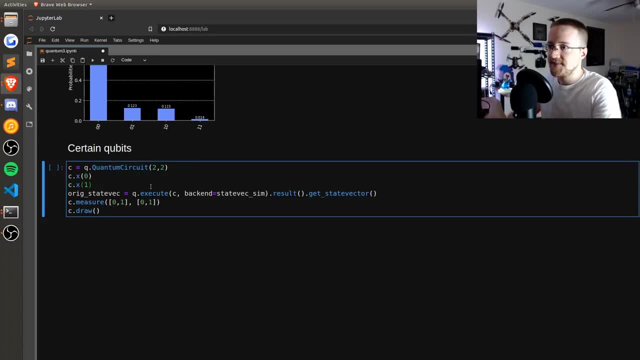 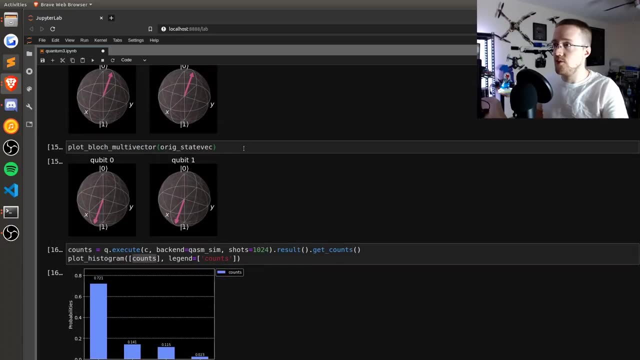 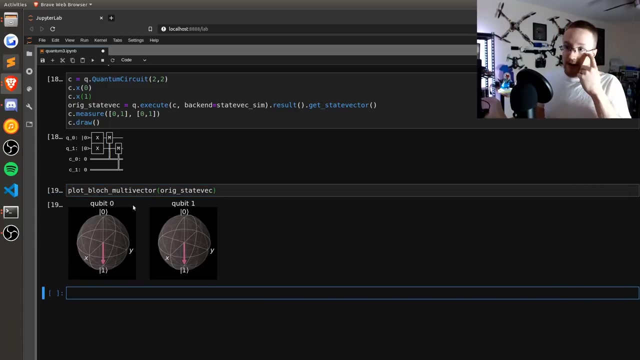 okay. so so we'll just say cx and then cx here. so that's our um, what we've got now uh and then uh, we'll just do. we'll just take this multi or the state vector here. so now what we do is: let's apply a hadamard on so hadamard in front of certain qubits. 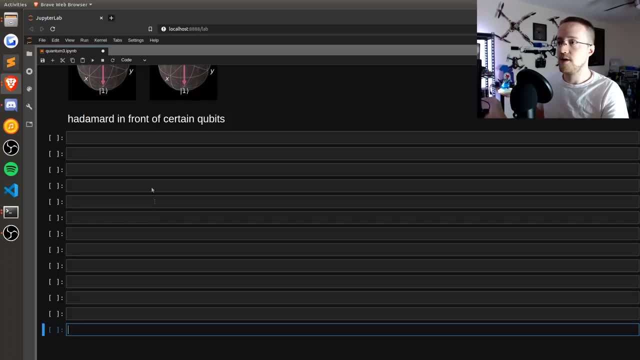 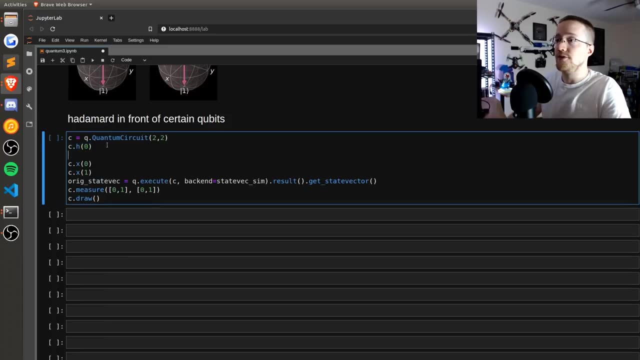 whoops, and then i'm going to make some space so we're not constantly dealing on the bottom here. uh, so now what we're going to say is c, dot, a, h, zero, and then we will do the one draw. we don't want to call this original state vec anymore. 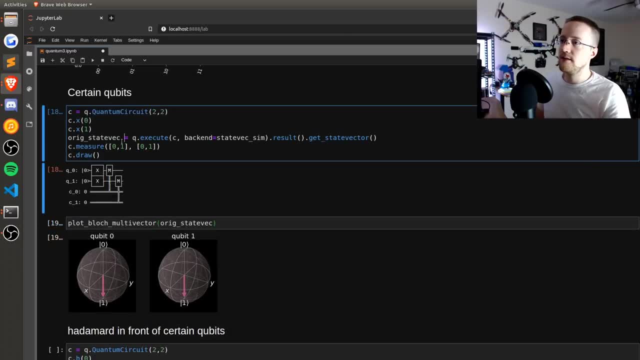 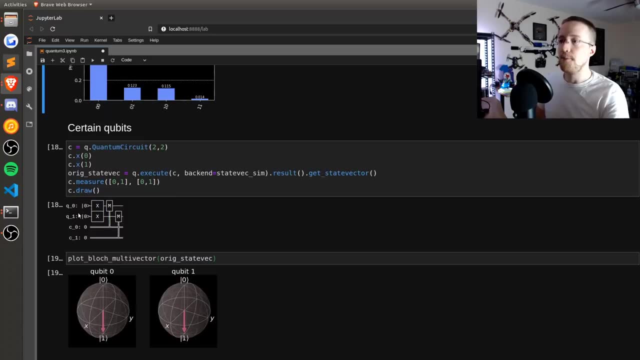 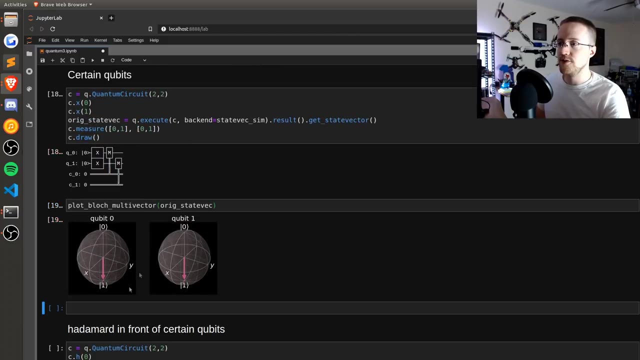 oh, i kind of want to do the. uh, i'd like to do the original counts as well. let's go ahead and let's get that done as well. so let me, let me just pop that in here. so just b for bottom. uh will give us that. so those are the. i guess we'll do the vector and then we'll do this. 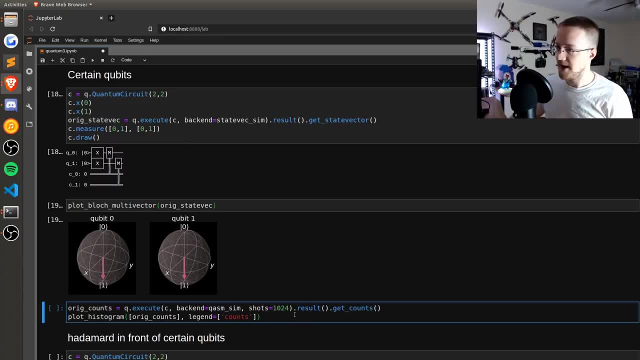 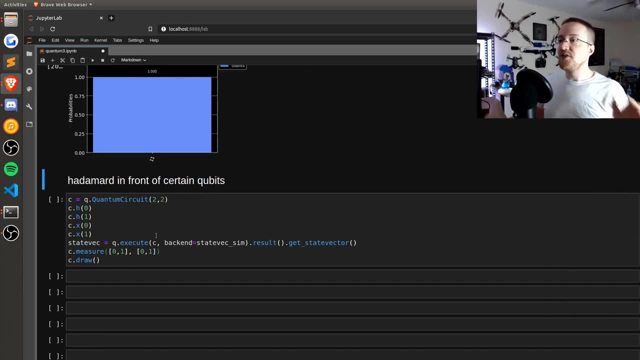 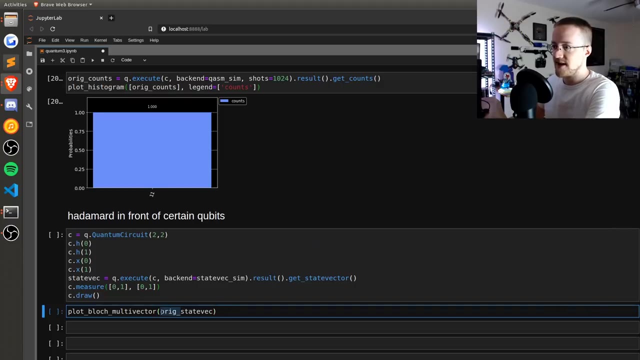 i should give it to us. let me just i'm let me make sure i haven't made some sort of silly error here. we should just get one, though, right, so? so we always get a one one, okay? so then we throw a uh hadamard in front of everything and then change this to be state vector. 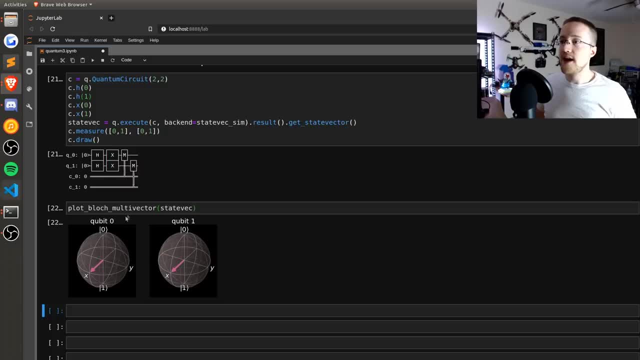 so so we'll run this circuit, cool. so now there's hadamards in front and now we've got this sort of situation where it's like just fully pointing towards that x. then what we're going to do is, let's look at the counts now. i mean, you should, you should kind of know what, what to expect. so 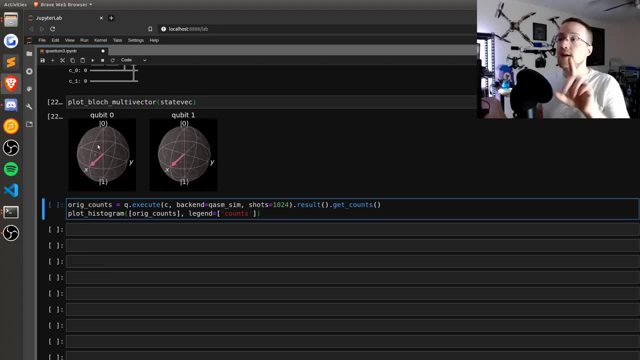 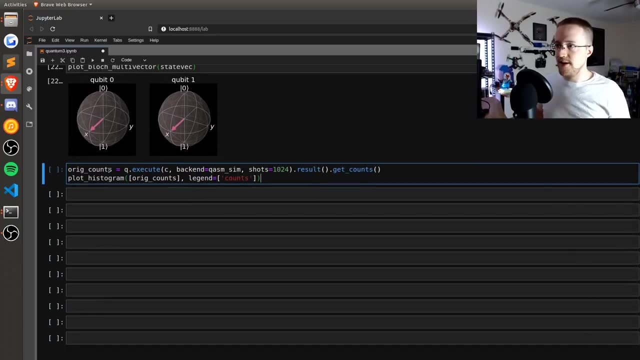 again, like i've tried. i've tried to kind of do this every time, but applying a hadamard to, let's say, a not gate, what do you? what should be the distribution output here? so let's see a ridge: counts, just counts. whoops, cool. so it's what you hopefully expected. right, it's just a. 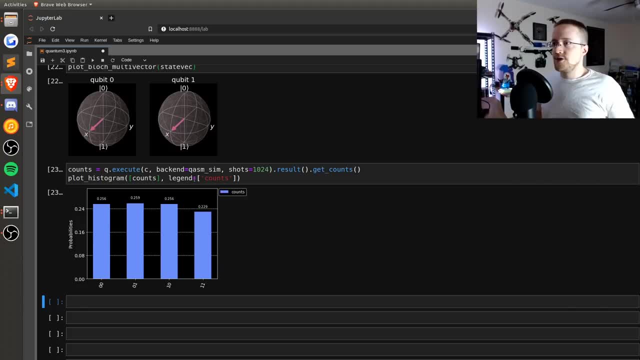 perfect distribution of all the possibilities here. so again, don't forget- this is a point where i want to stress- that in order to get that distribution, we had to take many shots right. we had in order to know that this circuit, like if we couldn't look into this circuit in order to know what the distribution this circuit had. 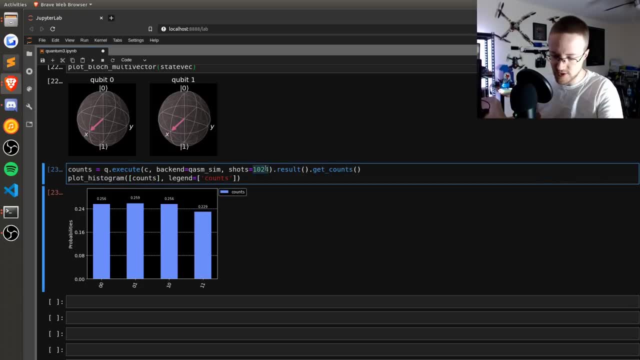 like. in order to know that characteristic we had to take a lot of shots. so if i just said one shot here we get one, one type of result. this is not informative to us as to the um characteristic of of the circuit. okay, so it just happens to be the case that when we take 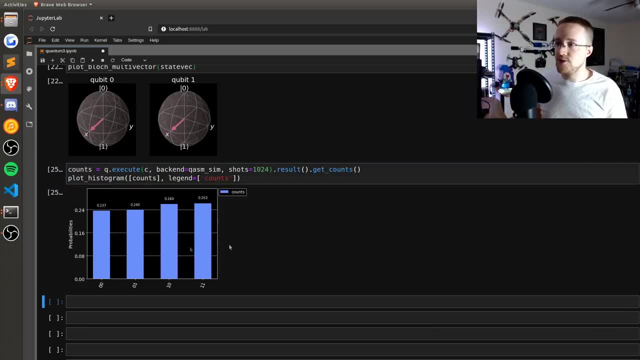 many shots because of the superposition state. here we get a distribution, but what we're building up to here is the ability to know a little bit about what the output should be based on- this hadamard sandwich. so, okay, back to what we're doing. so we've got hadamards in front right now. 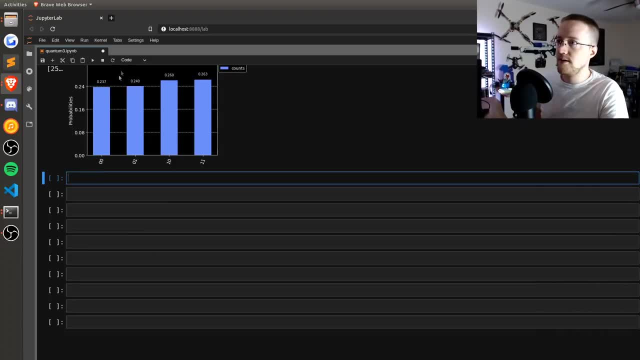 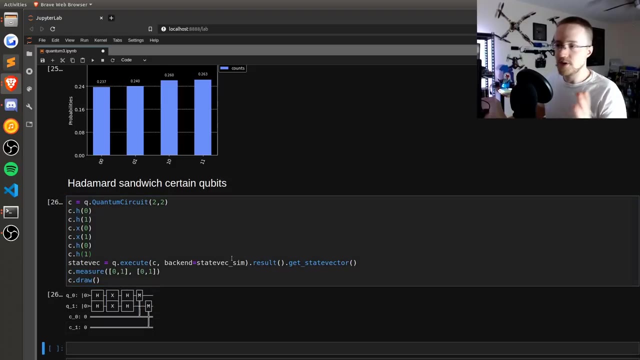 let's do a hadamard sammich, hadamard sandwich sandwich, uh, certain qubits, so we paste that in. and then, hadamard, zero one had them on zero one. draw, the circuit looks correct. nice little sandwich going on there, uh. and then we will do our multi-vector. okay, now, that is the on. 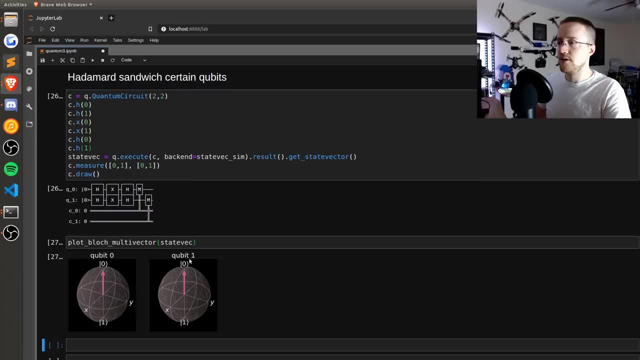 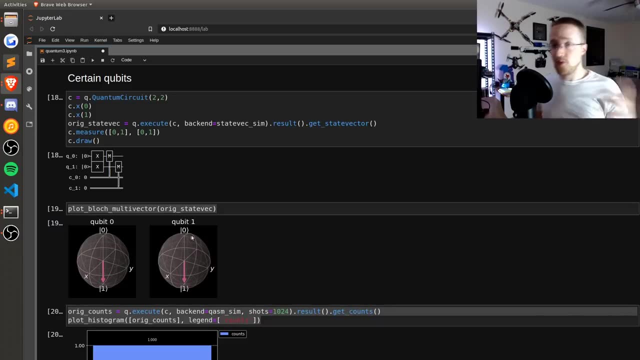 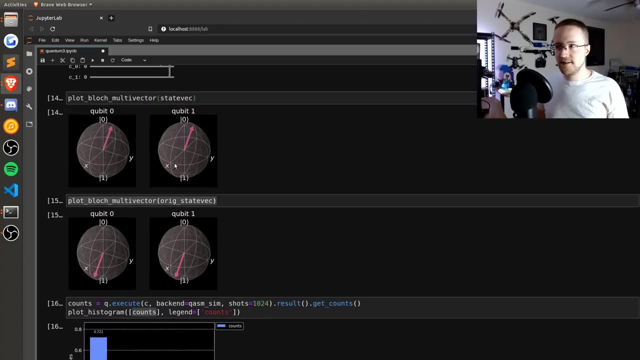 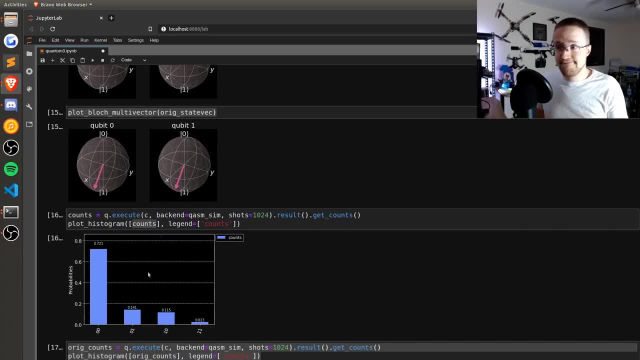 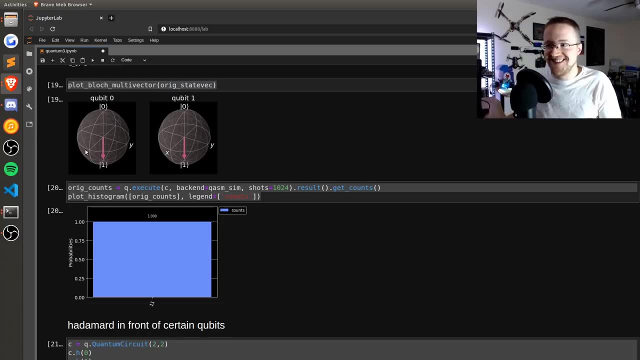 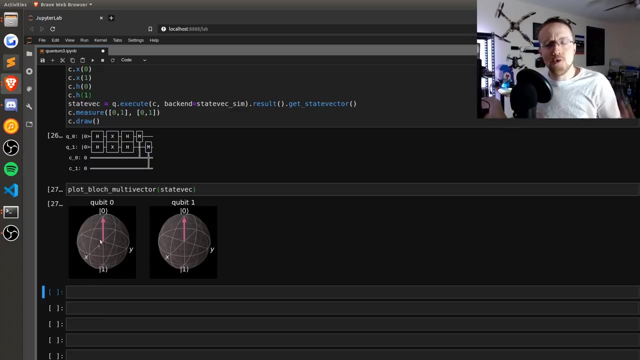 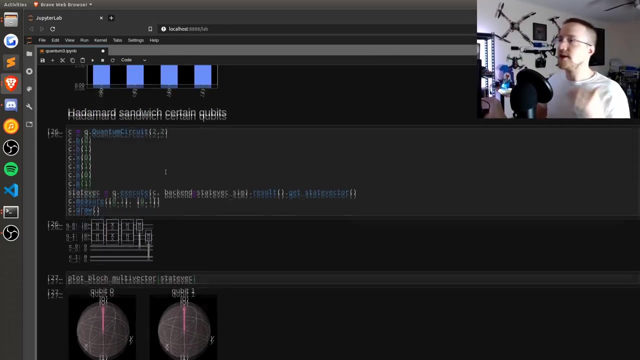 should have collapsed mostly to one one, but it doesn't. but coming down here, this should collapse, right. um, oh, it's flipped, so this should collapse to zero, zero every time, right, like. if this doesn't, i quit because i have to work in some. i have to work at least with some. 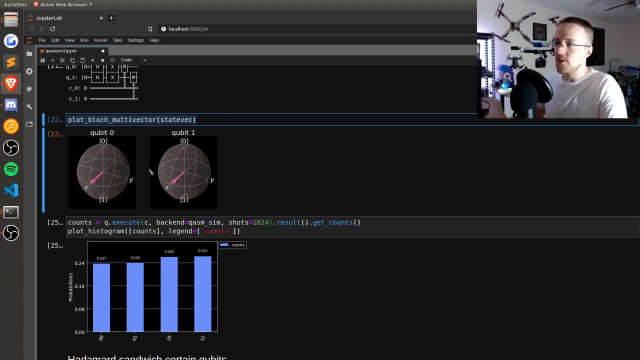 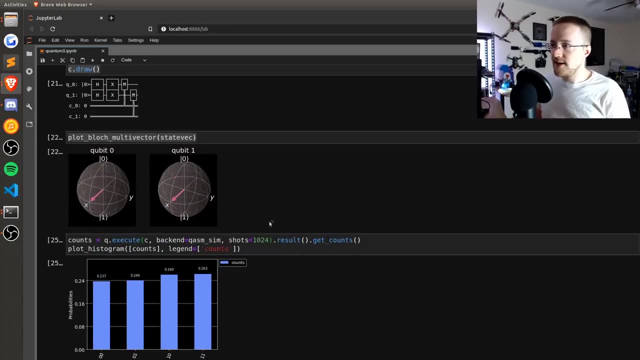 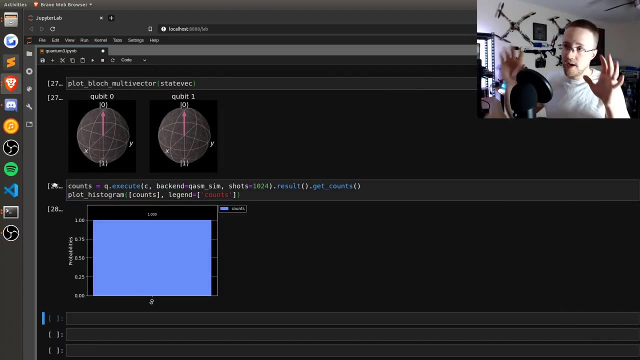 rules. okay, i understand, some of these things are kind of funky, but come on, without rules, what are we so savages? so, oh, we already plugged the multi-vector. what i want is the counts. so we come down here and we do the counts. now, this is our hadamard sandwich on certain qubits, and what we do get in this case is actually flipped values. 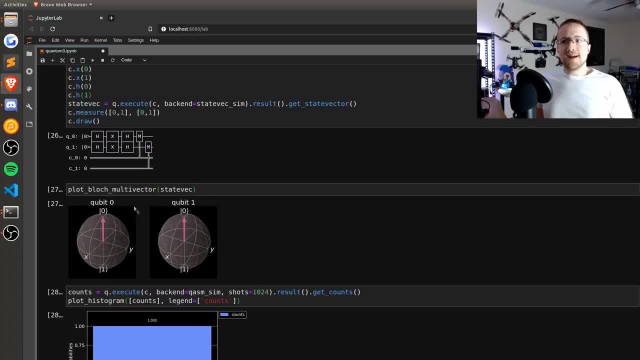 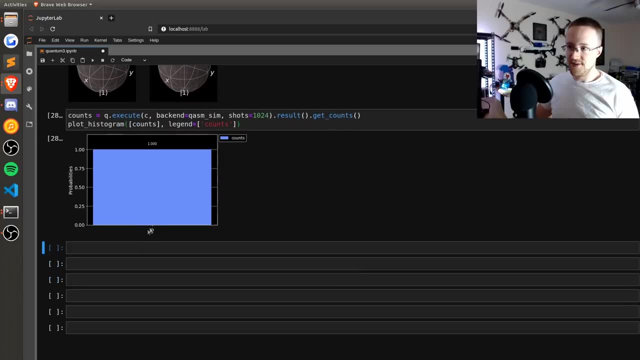 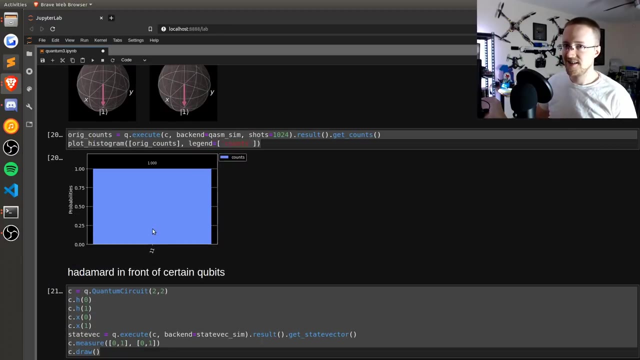 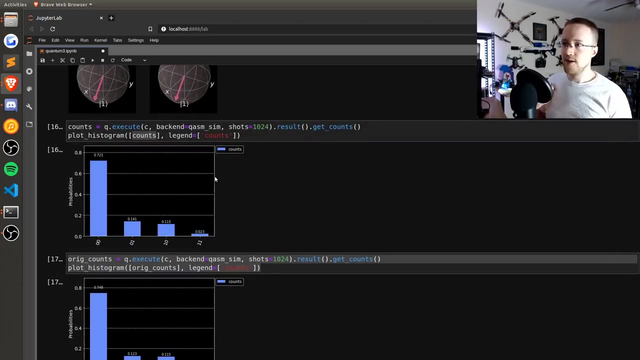 okay, which is still pretty interesting behavior, and it's important to take note that a certain qubit will respond in this way and an uncertain qubit will respond this way. so what does that tell you? so, getting back to our deutsche algorithm, this tells me: oh, we can do something interesting here. we can take 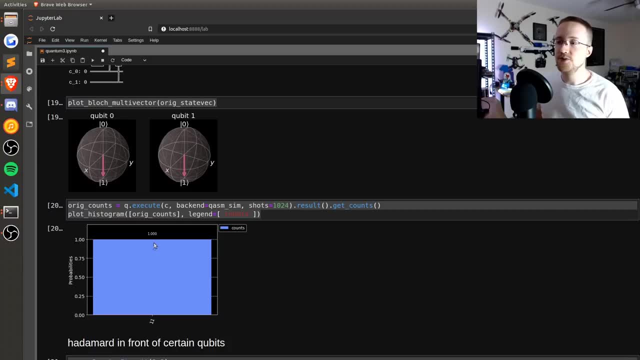 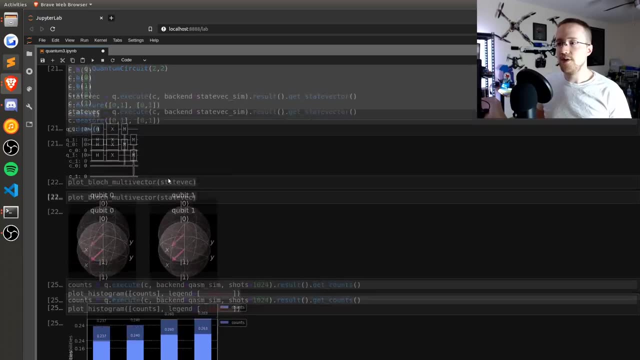 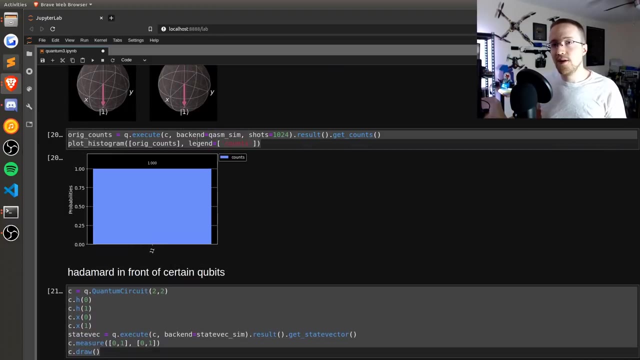 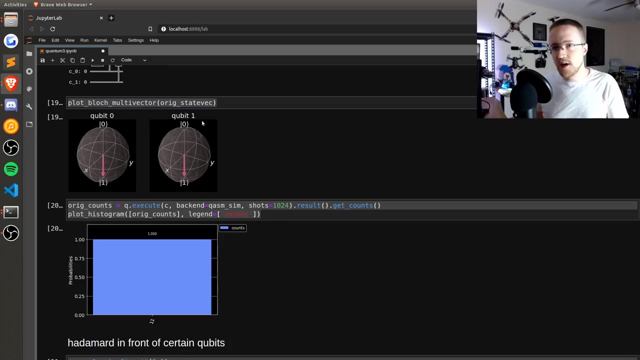 probably any n number of bits. use a hadamard sandwich to determine: is our algorithm or is our like little box here going to return to us um variable output or not? now, if we just have what we have here without understanding the inputs coming in um we would, we might still see things getting flipped. 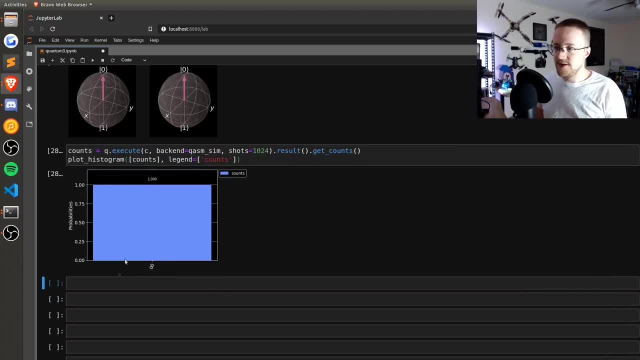 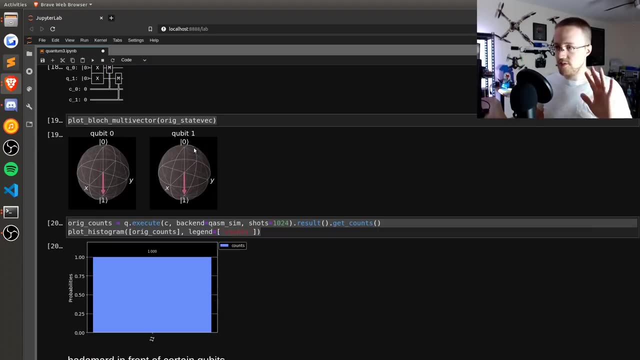 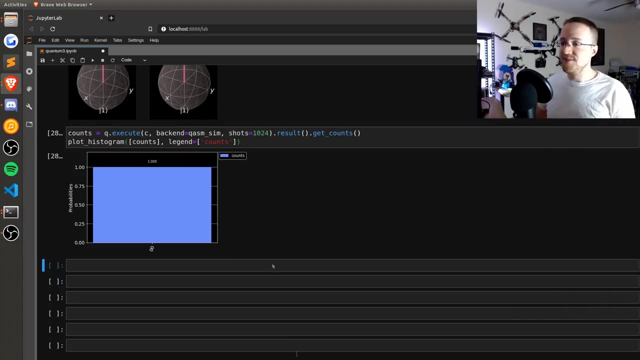 but this is the very, this is the basis right away: zero, zero for a constant one, one for balance. so keep that in mind. you've just been shown something amazing. so now, um, now that we've done that, what i want to do is propose to you, uh, the the rest of the. 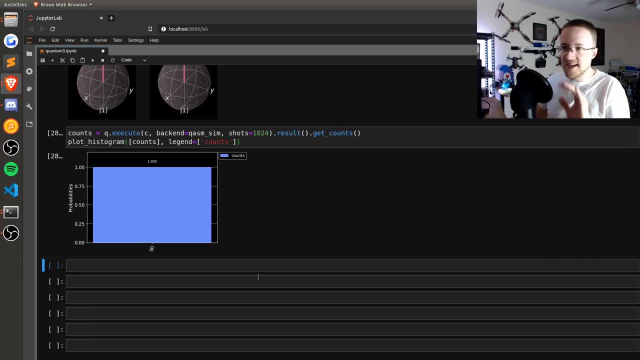 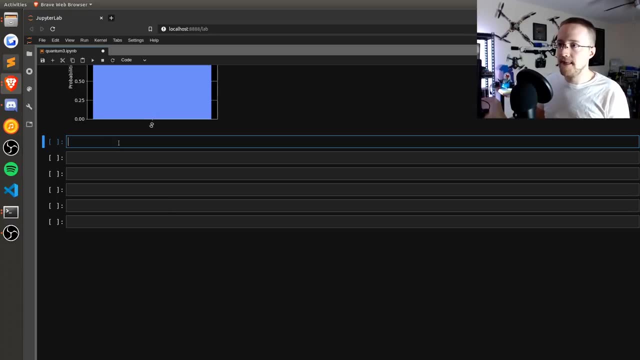 deutsche algorithm, because i think a lot of this gets lost when people just go straight to the deutsche algorithm. now, everything i've shown um is still applicable and it's part of the deutsche algorithm, but usually you just get it coded all the way through and that's not the point. 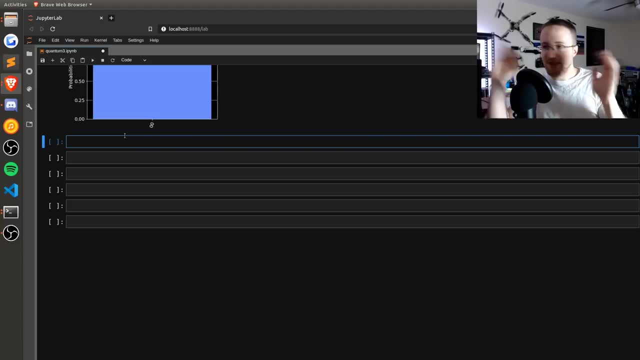 or people focus on the black box. that's not the point, that's not what's cool, like that's it. that's that has nothing to do with it. so, um, okay, so now let's go ahead and define our black box, um. or actually let's say a balanced black box. it's going to take in a circuit and it's going to output a. 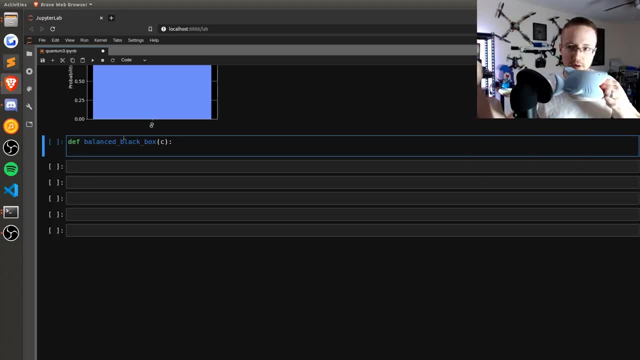 circuit. so we're going to make our little black box function for balanced and constant, so, um. so let's go. so for constant, what i'm going to do is make this for um in the way that everybody else has presented the deutsche algorithm. so we're, the black box is: 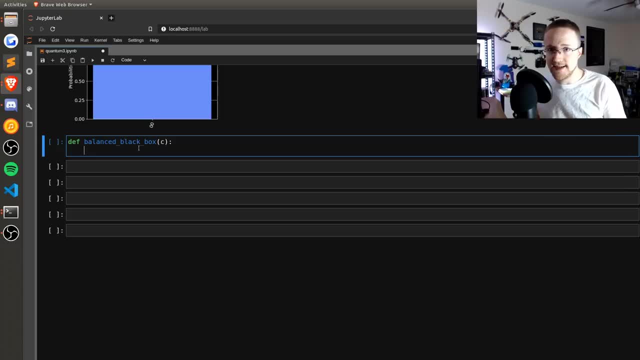 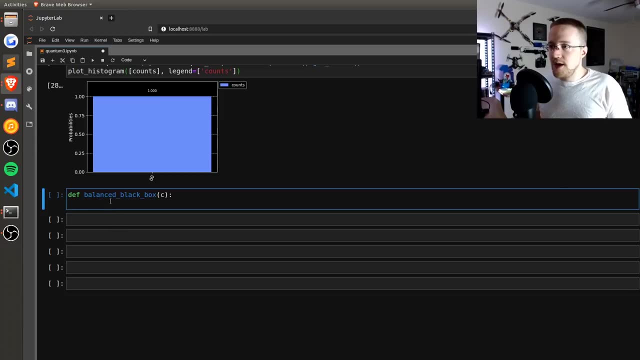 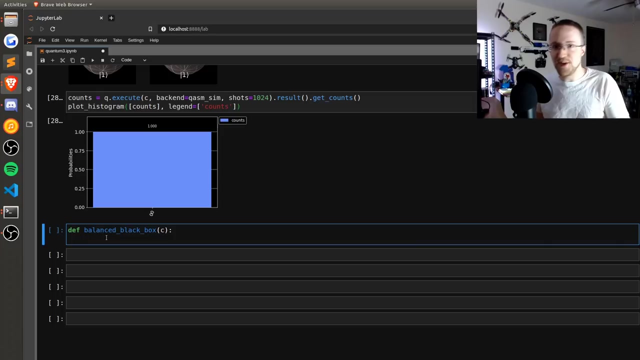 this balanced? uh, either balanced or constant, and the way everyone does it is with the controlled knot, so i'm going to use it with a controlled knot, but understand, there's so many other things that we can do here. uh, besides just the one way that the deutsche algorithm is formulated and 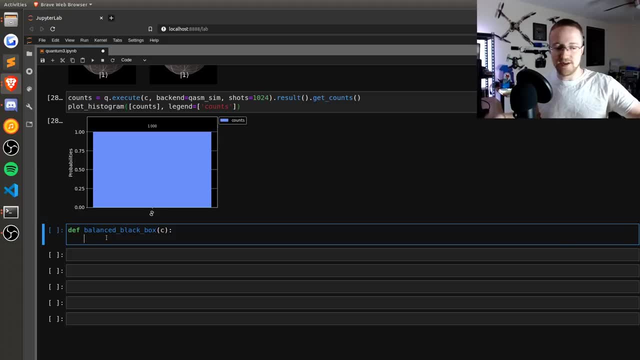 this is why the deutsche algorithm is is the basis for all these other algorithms. it's not like people actually care to determine whether a quantum circuit is balanced or constant. it's that we can determine that all in one pass, because that one pass can consider all of the possibilities. so 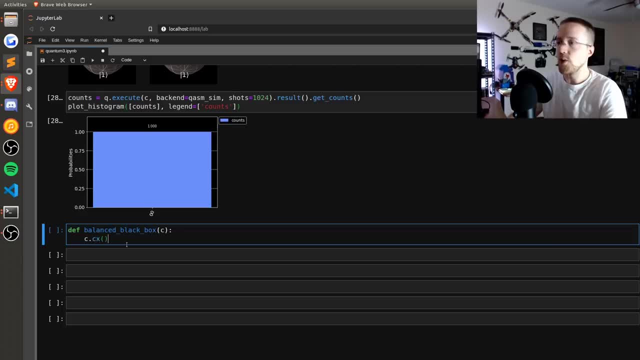 anyway, we are going to use what everyone uses this way. if you are confused, i thought about not doing the typical formulation, but i feel like with a topic like this- at least for me i've been- i've just been scouring the web for just all the resources i can find, and then i'm looking to compare things and just see. 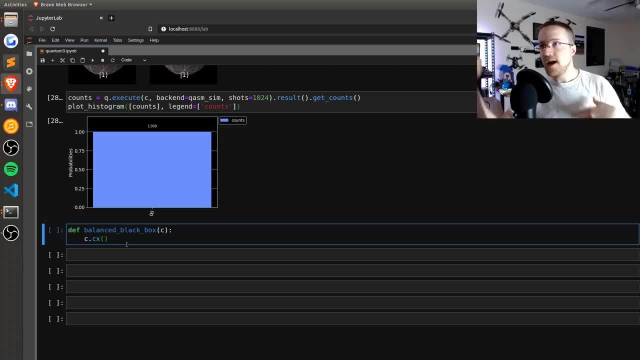 like see how one person explains something, how another person explains something like in the learning process, it's useful if everyone is at least using sort of the same things. so i'm going to use the same things, but just know that the possibilities here really truly are endless. you 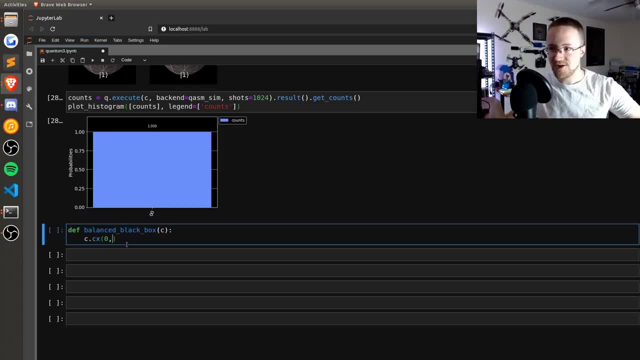 don't, you're not going to use the same thing, you're not going to be able to use the same thing constrained to this formulation. So, anyway, we're going to do a controlled knot from the zeroth to at index 2, which you'll see in a moment. We're going to add another qubit here. 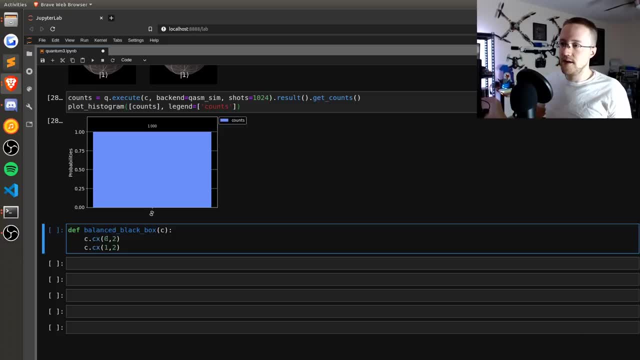 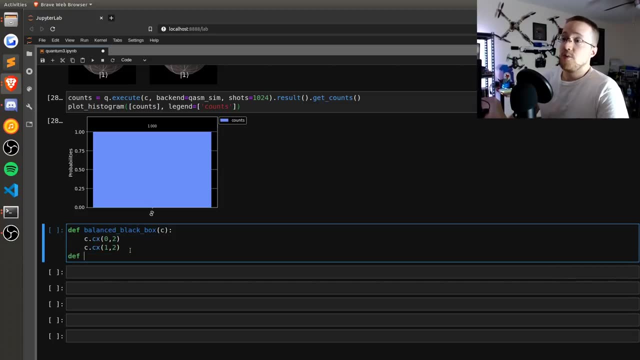 So we're going to do this entanglement between qubit 0, qubit 1, and they're just going to entangle with this qubit at index 2.. Then we're going to say a constant black box. It's going to take a circuit. Oh, and this needs to return a circuit. So we'll just define our. 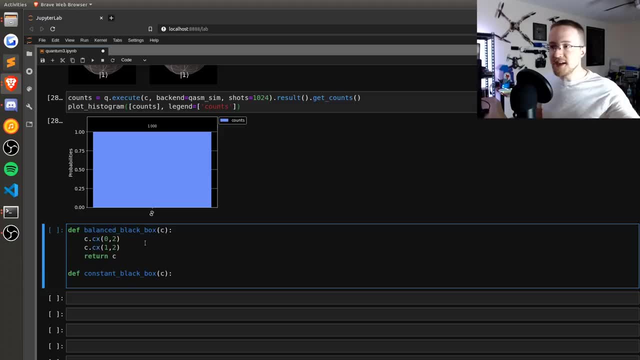 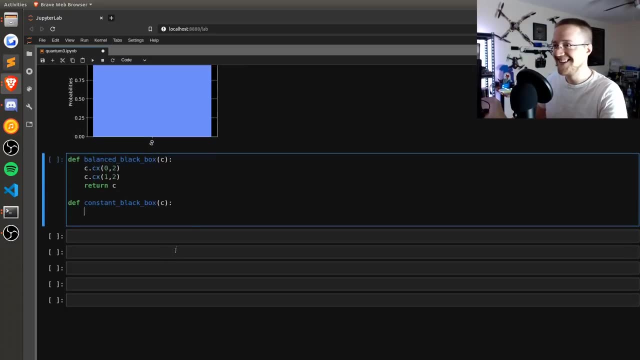 circuit and then, when we're ready for this black box, we'll just c equals c, basically, or c equals black box c. Anyway, you'll see Pun intended. Okay. so the constant black box, the easiest constant black box, is to just return c. 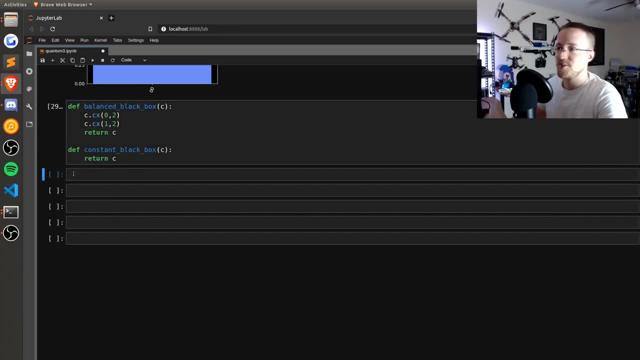 We don't got to do anything. We don't got to do anything, So expert tutorials, Okay. so now what we're going to do is we can define our circuit now. So we're going to say: c equals quantum circuit, and again we're going. 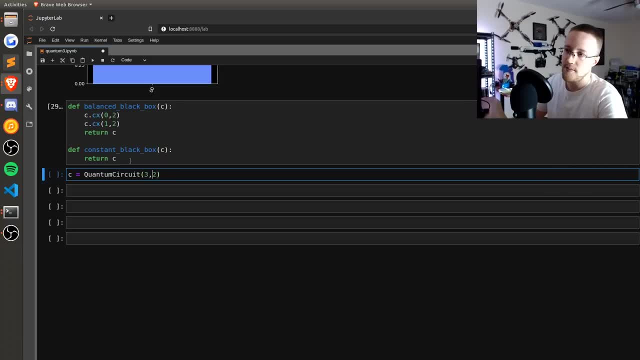 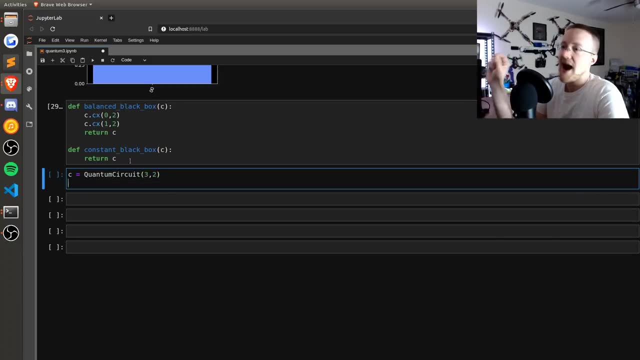 to have three qubits, two classical bits, because we don't actually care about qubit number. Well, qubit at index 2.. That's not relevant to us, because instead, what we're actually curious about is what are the outputs to qubit? 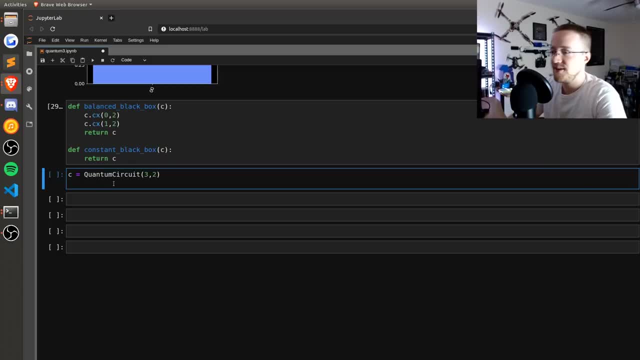 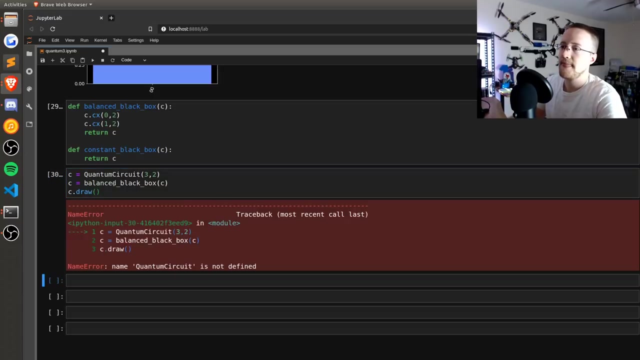 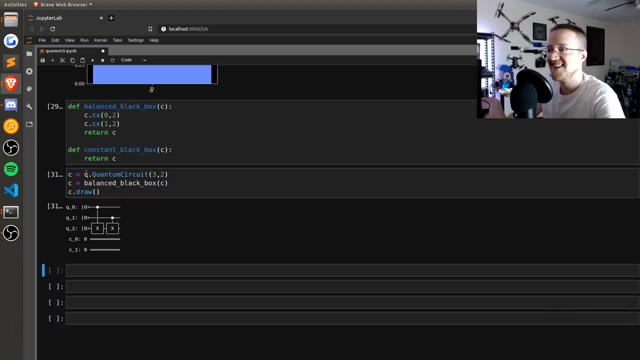 One and two, So anyway. so what we're going to say now is: c equals balanced black box c. So now, if we did cdraw, cdraw, quantum- Oh, I keep forgetting the stupid q. I'm pretty sure I spelled that right. Okay, so, as you can see, we started it. We can apply this. 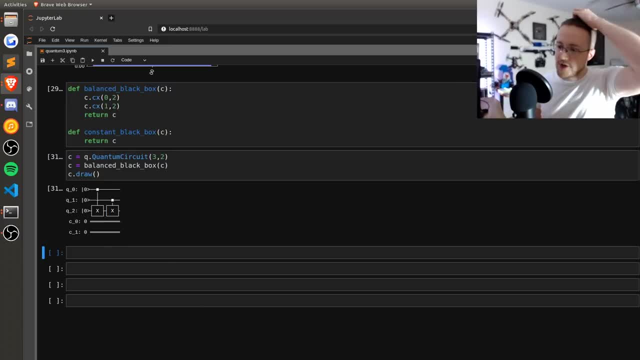 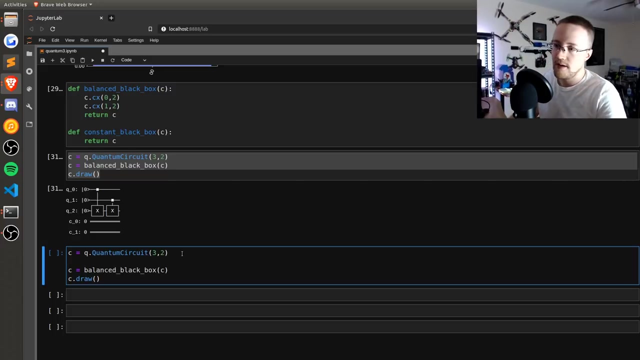 black box, however we feel. So now what we're going to do is encase this in the Hadamard sandwich. So we're going to say basically this: copy paste, and then we're going to apply Hadamard gates to basically everything. So we're going to say ch012,. 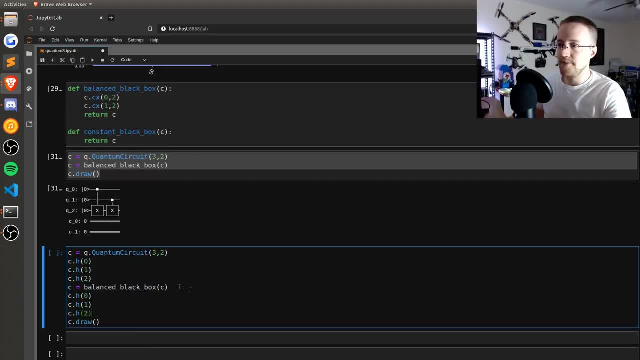 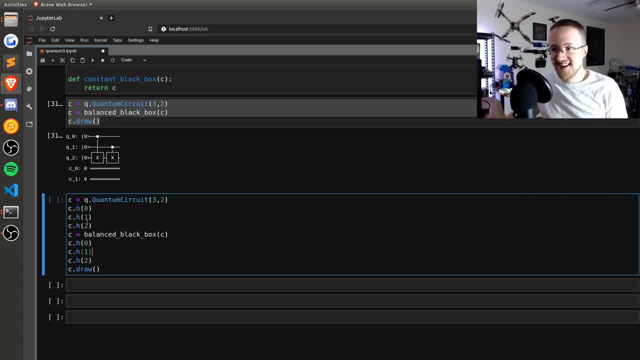 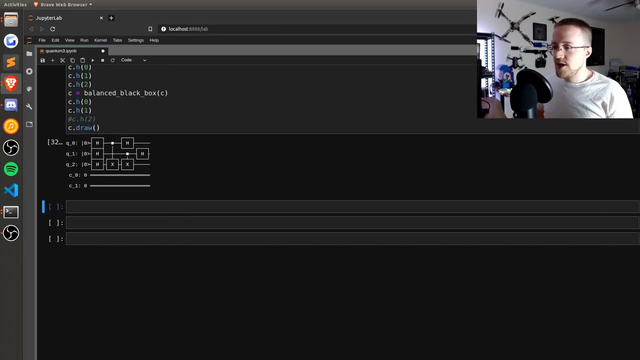 but you don't actually need the Hadamard gate here, right, Which will make more sense later on. You can put it there for symmetry if you really want, but it's unnecessary. So now what we have is the following circuit: So things are starting to get kind of jumbled up. So one option you have. 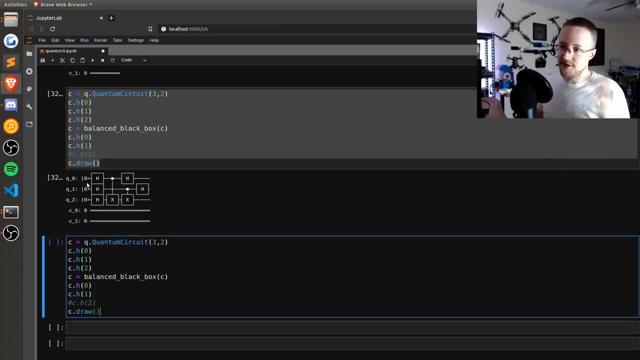 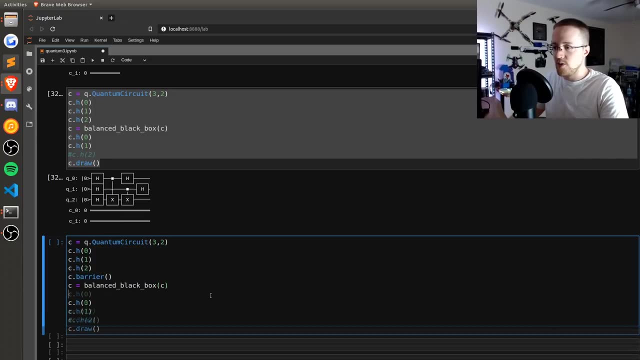 when this is happening, especially if you're just trying to make things clear- is you can use this barrier. So, for example, you could say cbarrier, and it will create this little line for us. So just a quick example here: Run that and so now you can see it's a little easier to read, right. 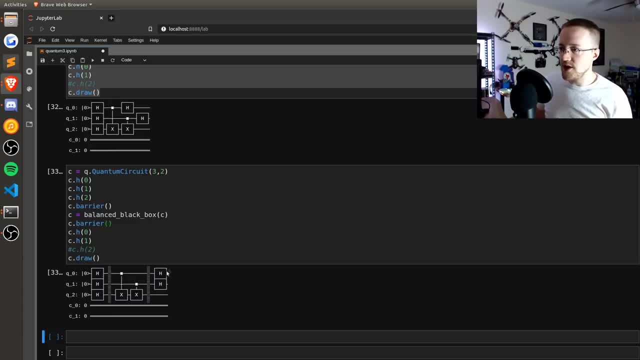 It looks a little more linear as far as what's happening At this point. you could Hadamard over here Like it's totally possible and it's fine, but it's hard for us to read it if everything's not in line. So as far as I can tell from looking around, 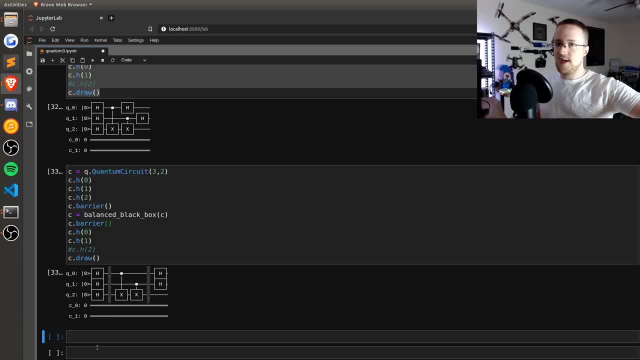 the barrier is used to stop the Qiskit optimizer, like in the back end. that optimizes your actual input circuit before it goes to the quantum machine That will optimize your circuit. So if you're doing something stupid and wasteful, it appears to me that they can fix that with. 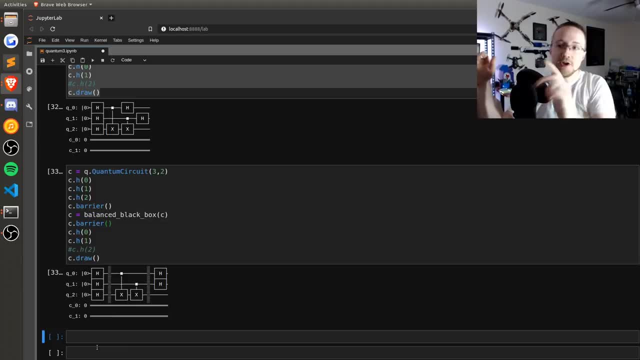 this optimizer, But so you can use the barrier to stop that from happening. So now the optimizer will optimize this section, this section and this section. Again, this is my understanding. I could be wrong. I see barrier actually being used. It's just purely for aesthetics, It's purely for making. 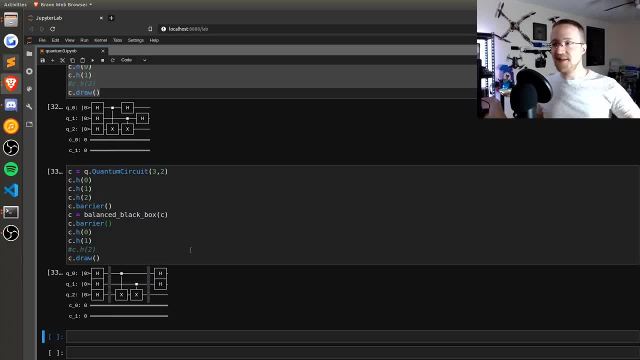 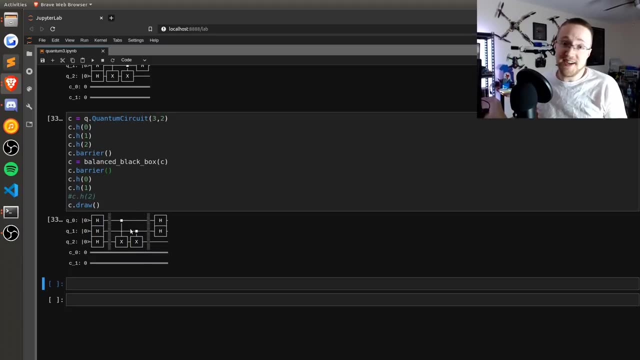 these easier to read. Maybe as I get deeper I'll find a scenario where I really need to stop the optimizer from doing something, but I haven't seen it yet. So anyway, like I say, I'm a noob, so maybe I'm missing it. Okay, So there's our nice, beautiful Hadamard sandwich. 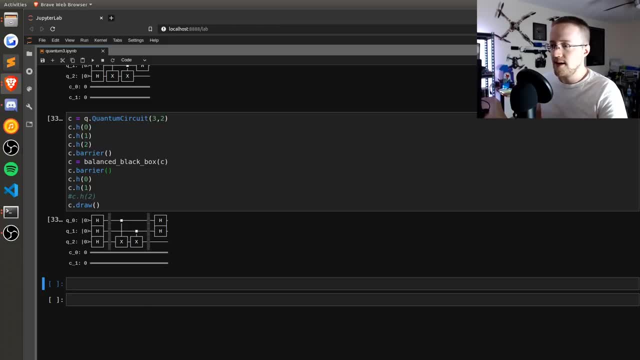 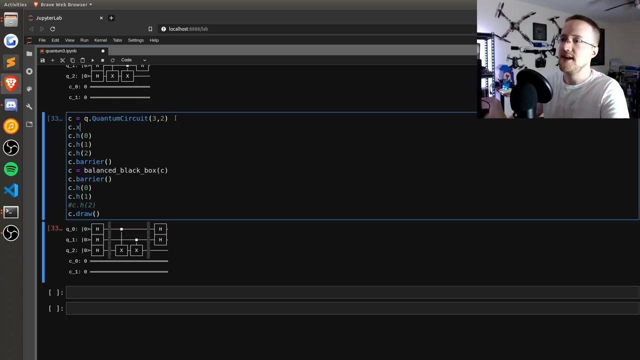 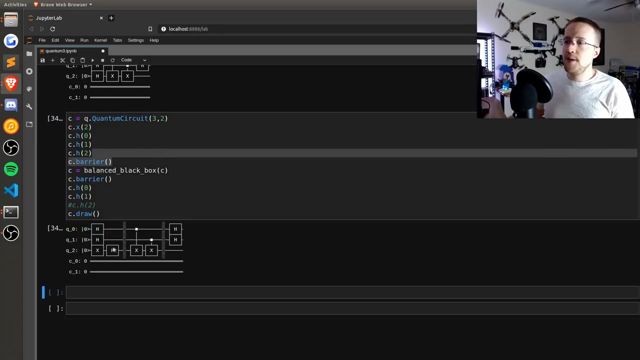 And I think probably. I think what I'd like to show before. So one of the things that gets added again to make this uncertain is: you can add what you'll typically see is a CX for gate two, So a not gate on quantum gate two. But before we just throw that in there, I want to talk about what that does. 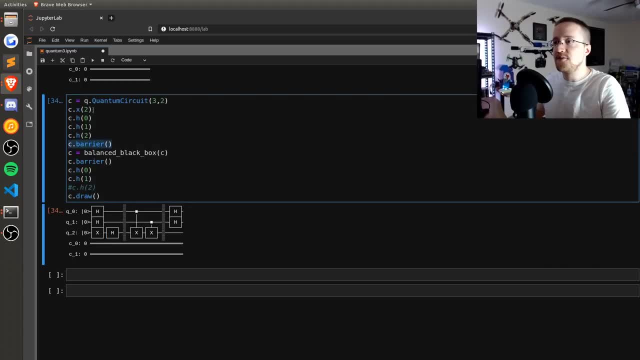 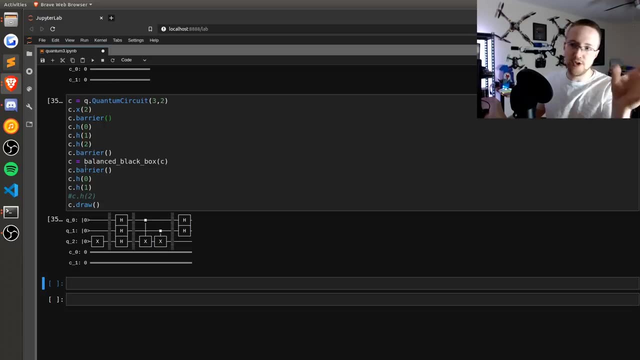 right, Because again it's kind of missed, And in fact before, exactly why we want to use this gate. So again, here's our little black box And if you want to be abundantly clear you can put like two barriers or something. but I think this is fine. 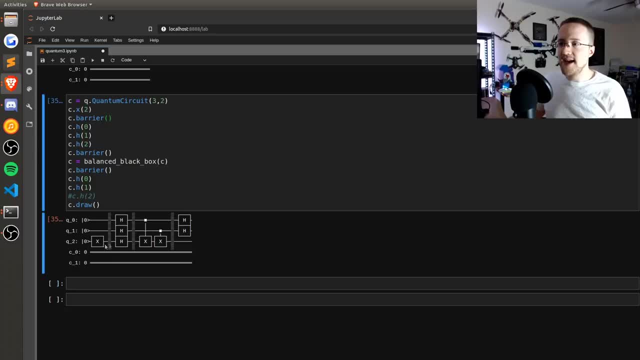 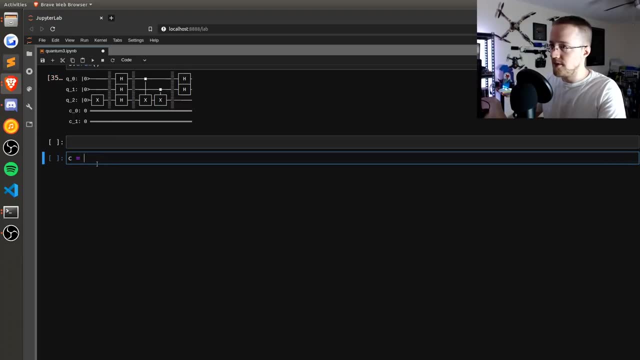 So what happens when you have a not gate and then a Hadamard gate? what goes on there? So really quickly again, I'm just trying not to gloss over anything at all here, because I think I think that, from what I've seen, at least when I was going through tutorials, I'm like trying to 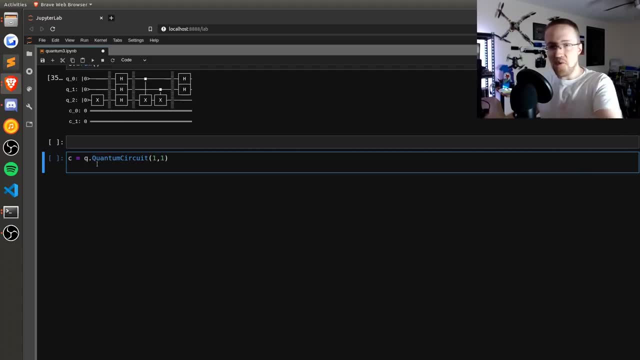 figure out okay. well, why is every single gate? Why are they here? What are they doing? And there's really not explanations for this. And this it just. it reminds me so much of why I started doing YouTube tutorials and in general like on on, just in Python, Cause I was like: no, you have to explain. 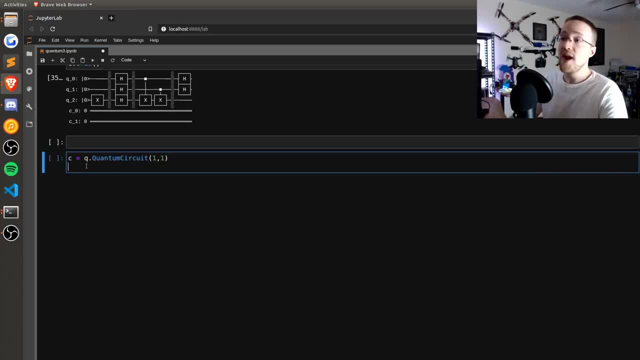 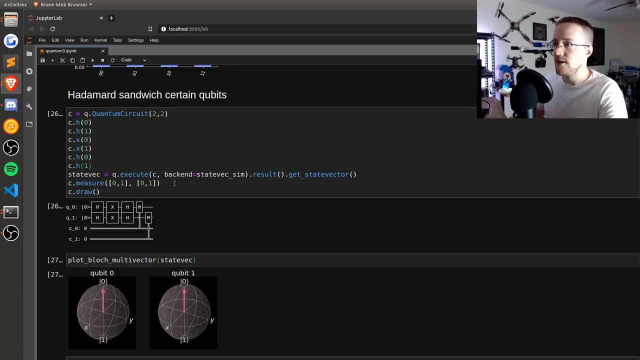 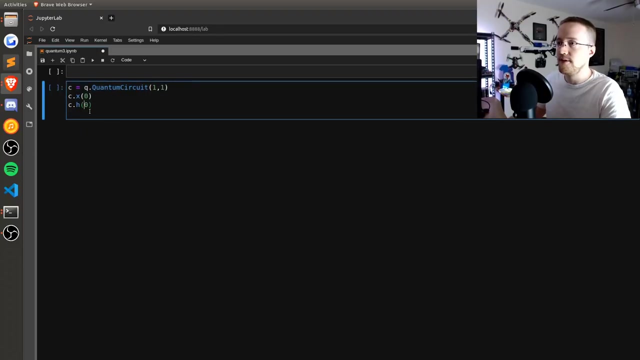 everything. You can't just skip things. So, anyway, what happens? Like let's see what happens when we have a, a, a, not gate, followed by a Hadamard gate, Whoops, So let me just, I just want to steal our state back. code: Stay back here, Come down here, Not that. 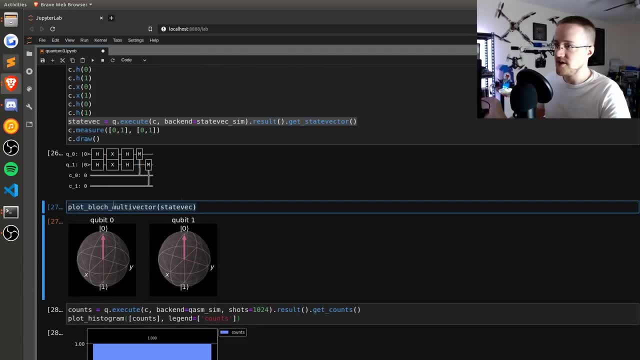 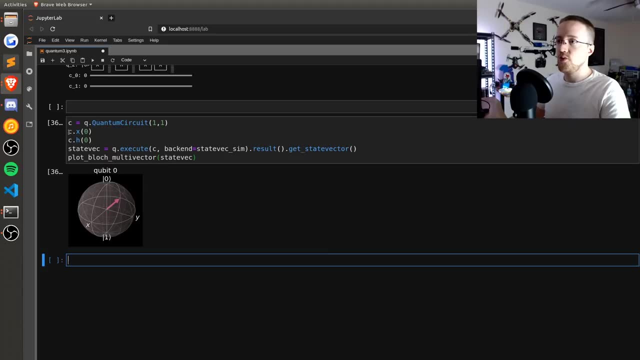 you don't have to follow along on this step. If you don't want, you can just look at it. I'm just trying to show you. this is all in the text-based version too, So don't worry about it. So, so what? 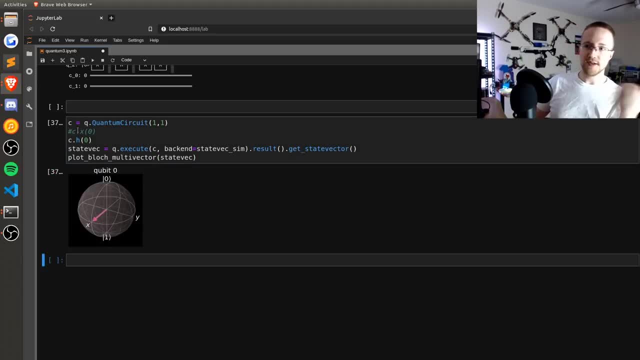 was the original Hadamard gate, right? It's this positive X value, right. But if we do a not, then a Hadamard, it's a negative X value. What if? what if we start with a Hadamard and then we, not the Hadamard? 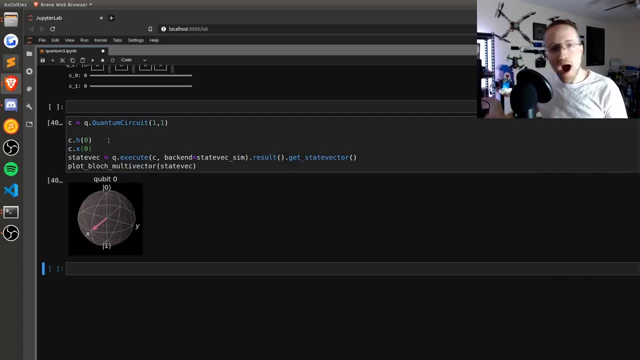 what happens, Not what we expected really. So now, what we're going to do is I'm going to ask a question that I'm hopefully going to remember to answer by the end, And that is: is there another way to achieve a negative X value? And I'm going to ask a question that I'm hopefully going to 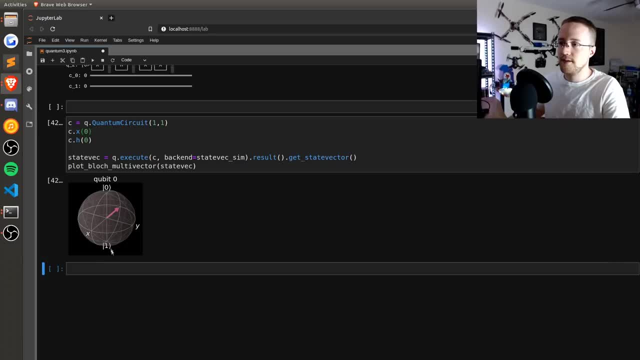 OR I'm not going to read, but I'm going to do it. And what are the reasons that the value baby that I have to do this is what's× × s× Times? half L of theações Ñ₂ ‧ó μα�üyorum. 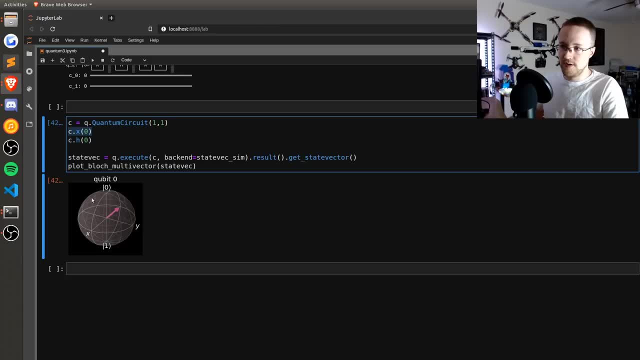 D. So what does it mean to achieve going from here to here? That does not involve what appears to be the requirement that you first have a, not then a Hadamard. Is there another way that we could do this right here? Think about that Cause again. the do chios algorithm is not specific to doing. 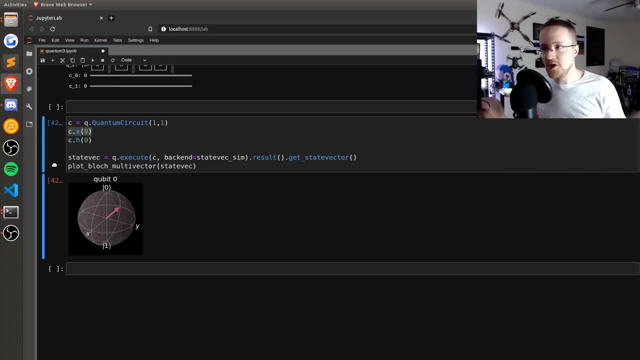 things in some perfectly exact way. Instead, It's there to show you that this, this characteristic, is on, like all of these quantum algorithms, when you use this notion of superposition. so think about it, feel free to pause it and think about or whatever, but at the end i'll show you. 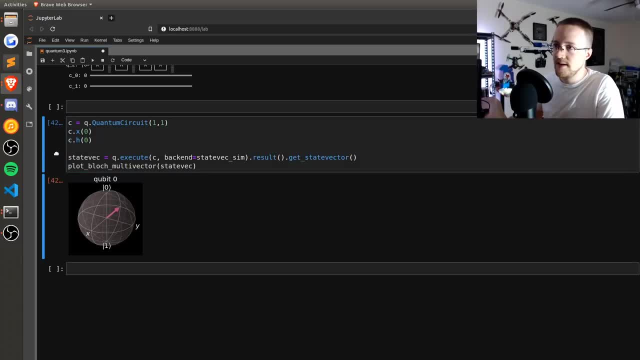 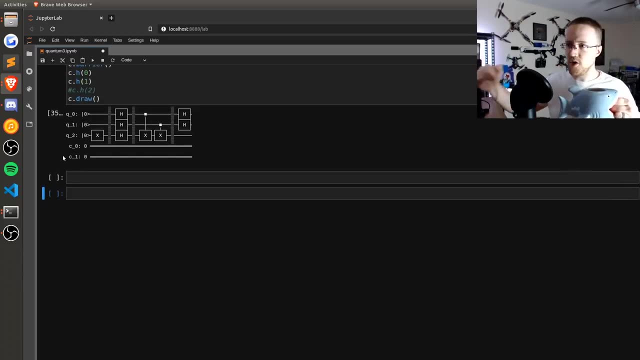 the answer to that question: will you go away? there you go. i couldn't get it to go away, like you press d, by the way, to get things to go away. if you want cells to the bottom be a top a like above, okay. so now that you understand what is happening when we add that knot, let's go. 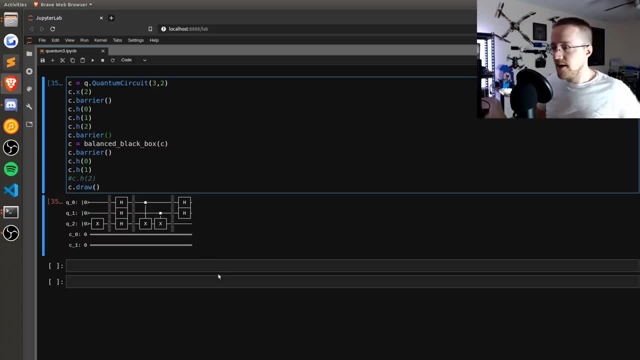 so we've already got it there actually, so we'll add that, not gate. um, i'm trying to think. i think we're actually, uh, completed here in terms of everything we need. the only thing that we need actually. well, we're our circuit is basically done, but we're not doing anything with the circuit. 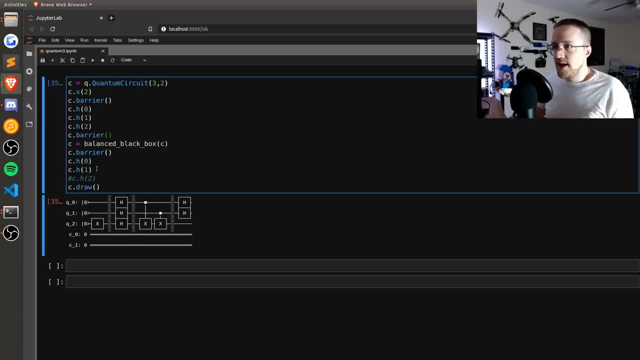 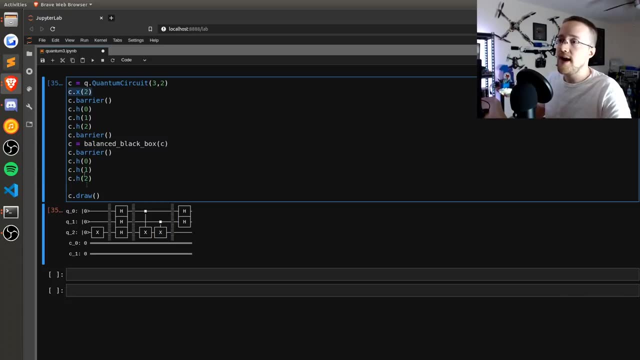 right? so, uh, let's go ahead and we'll take our measurement again. this had a market, you can add there. i have even seen people throw another x here. um, for the purposes of what we're doing. no, now, if you were gonna, maybe work with qubit. 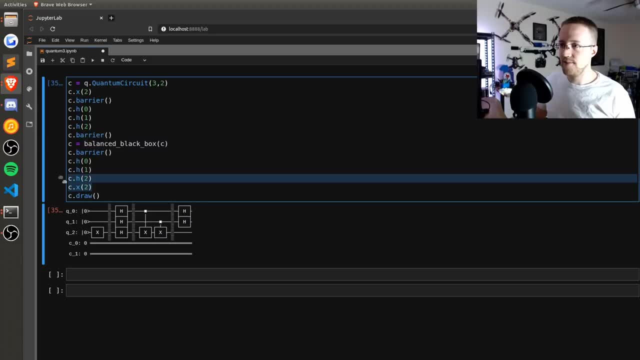 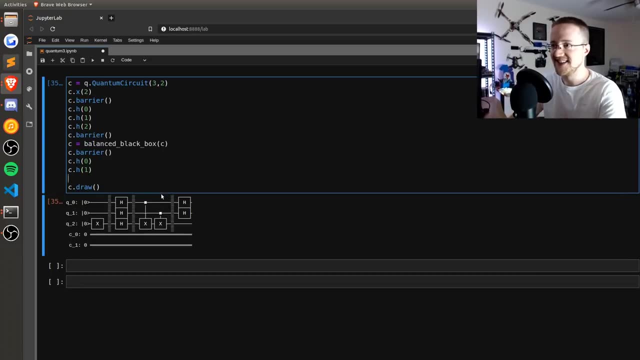 two at index two. you know, who knows what you might have here. but for the purposes of actually showing the circuit at work, no you, it doesn't have to be symmetrical, even though it's very, it is very, uh, tempting to make this a nice, perfect hadamard sandwich. just, i'm just saying 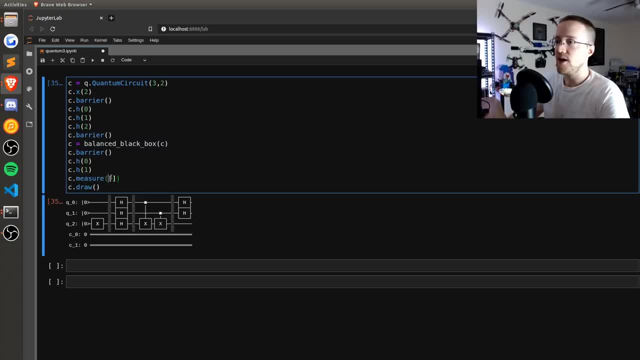 so now we're gonna say, c dot measure. and again, uh, we're gonna measure, uh, qubit zero, one, and we're gonna map that to, uh, the classical bits of zero and one. so here's our circuit. and now, uh, we can actually uh measure these um. so, uh, let's go to count. 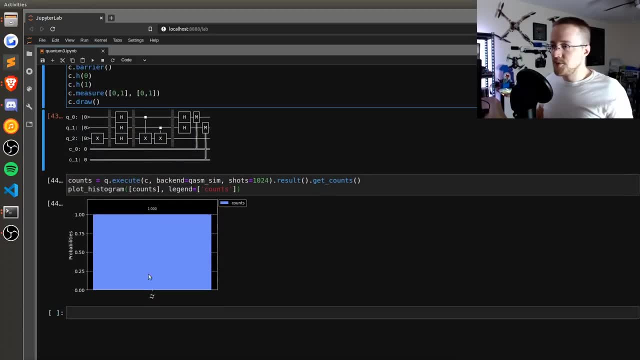 pasta. so what we get as our response here is one one. so it's not so what this is. what, basically, what this is informing us is? it's not really like the output to the circuit. instead, this one one corresponds to the nature of the internals of the circuit, or something it's responding to us. 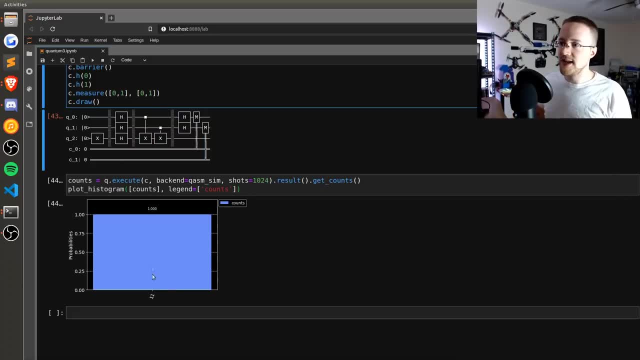 the nature of like the probabilities in the circuit. so in this case this is our balanced output. we're getting ones now. if you had, you can continue adding as many qubits as you want. so we've got two qubits here. you could have had 30 qubits if you had a machine that could do it. 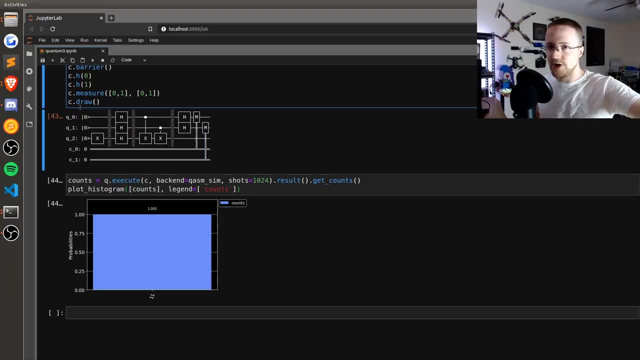 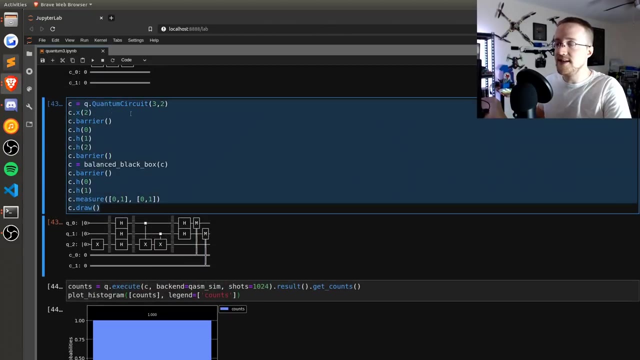 it's infinite. you can have as many as you wanted. you could answer this question of like what? what's the characteristic of this circuit in terms of is there balanced or constant output? so, continuing this, what if we went with, rather than the balance box? what if we did the constant box? 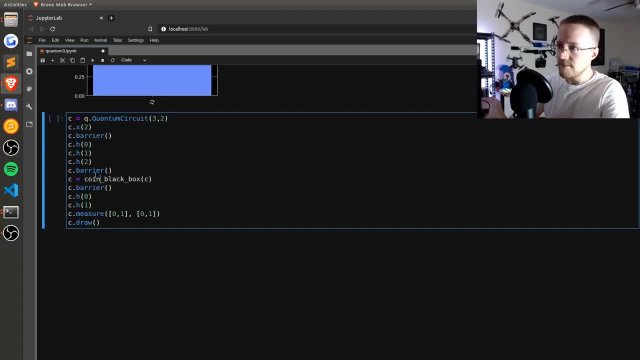 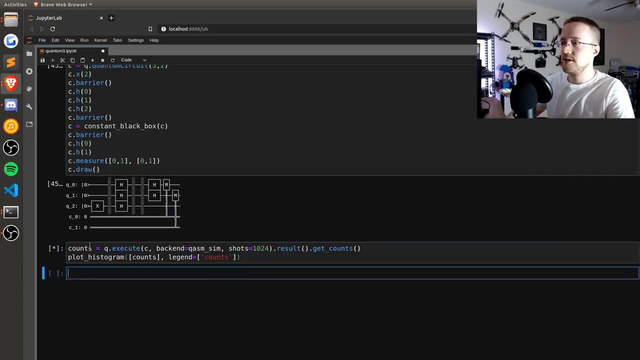 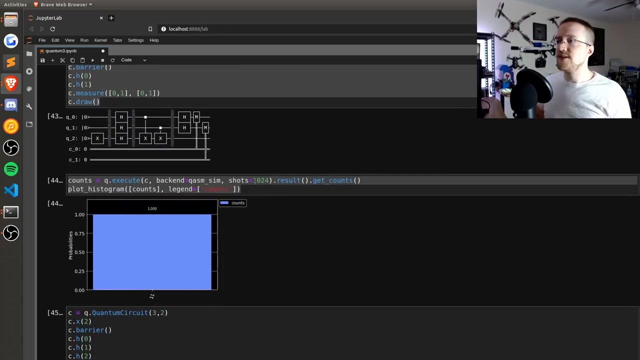 so i think we just called it constant black box, constant, yes, okay. so uh, now we do the counts, run that again, and what we get is zero, zero. and again- it's important for me, i think, to stress this- is one, one for every single shot. so we took a hundred. 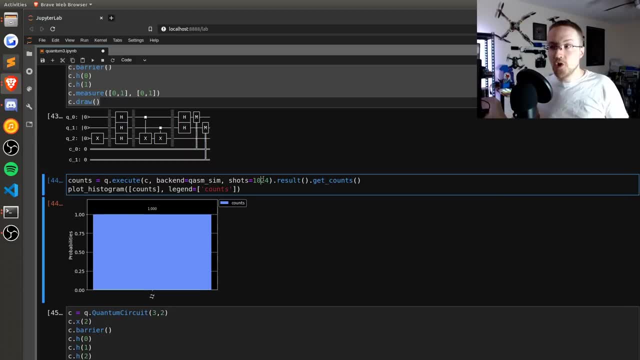 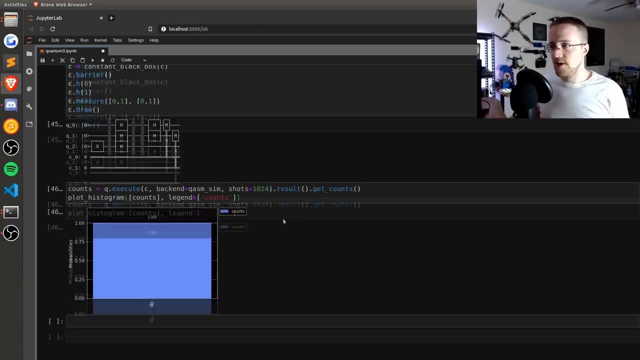 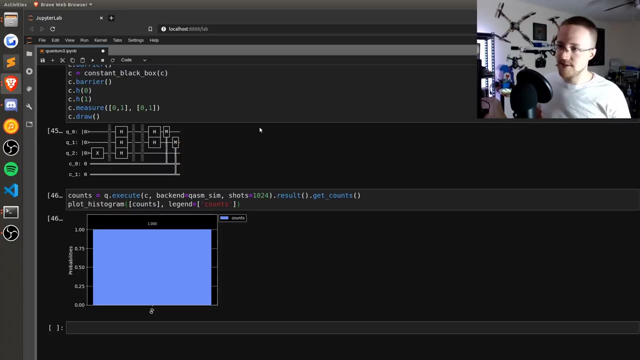 or a thousand twenty four shots, but we could have gotten this answer with one shot right, it's a hundred percent one, one always. so given a perfect quantum machine, we would have always gotten this response. of course, quantum machines, again, have noise, so we have to. we can't quite get away with that yet. 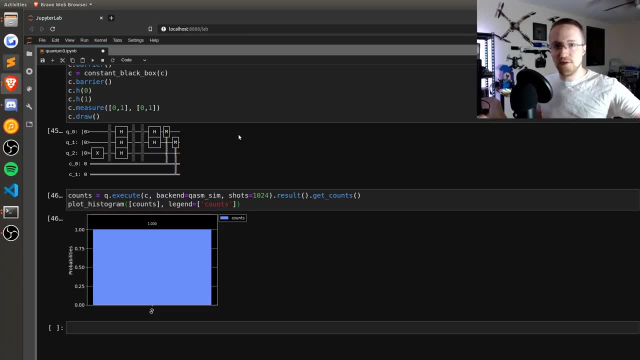 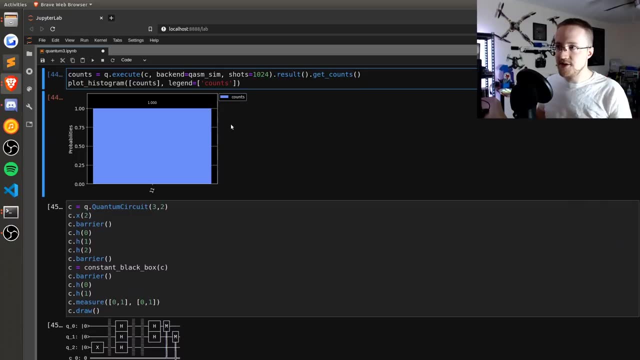 there's no reason to believe that i know of. we can't reach perfect quantum machines right, but again, fundamentally we can. we can query these quantum circuits one time and understand what is the variability of this output. that's incredible. it's just one shot through, but it's because of this output. 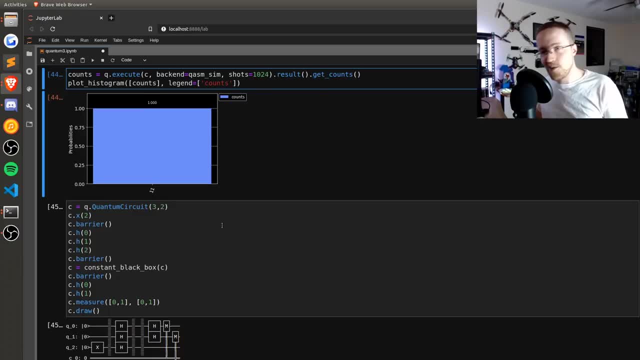 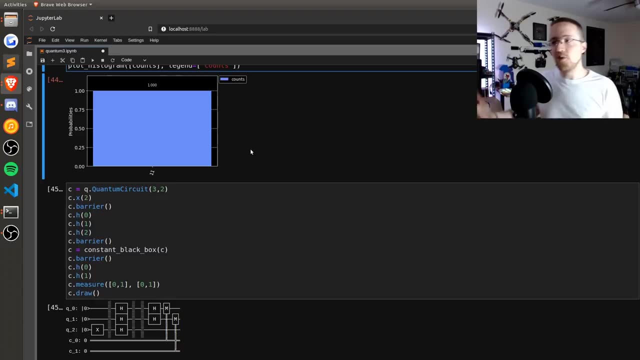 of this superposition and Hadamard sandwich that this can happen. right, So that's incredible, right. So again, what does this all mean? And like, where do we go from here? It's not really answering the question of: well, basically, this algorithm does two things, Like the: 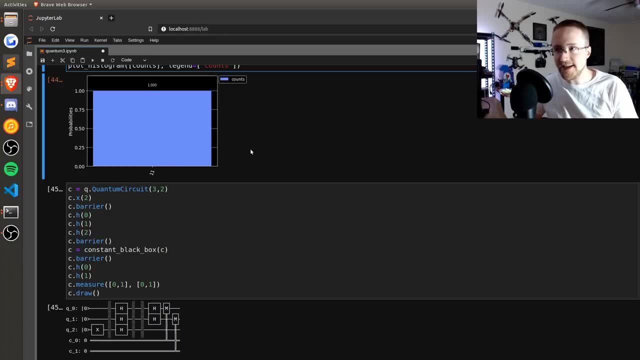 Dois-Josa algorithm is really the first algorithm that provably, like mathematically, can solve this question, even though it's a relatively useless question, It can solve this question faster than a classical computer. A classical computer would require at least two passes through the circuit. 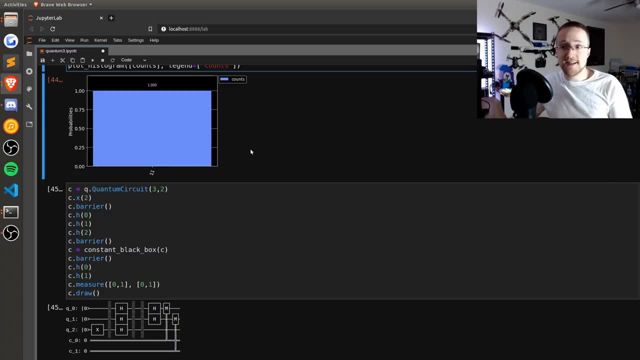 to answer this question. The next thing, and as you increased qubits, it would get even more complicated than that. So it's faster than a class, provably faster than a classical computer in terms of like how the cycle through the circuit. But then also what's more impressive, 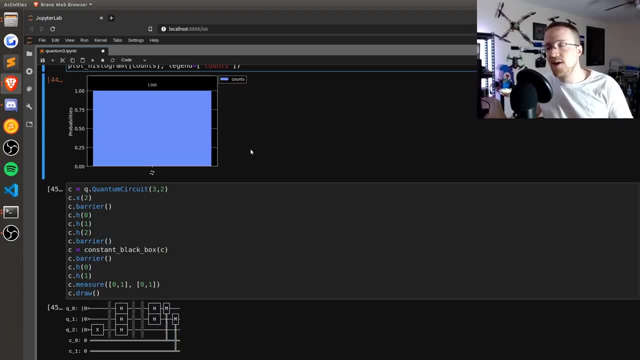 it's. it's like it's not impressive that it's faster. It's like: why is it faster, though? And we're like, oh cause we can actually query, while we're in superposition, the attributes of this this. 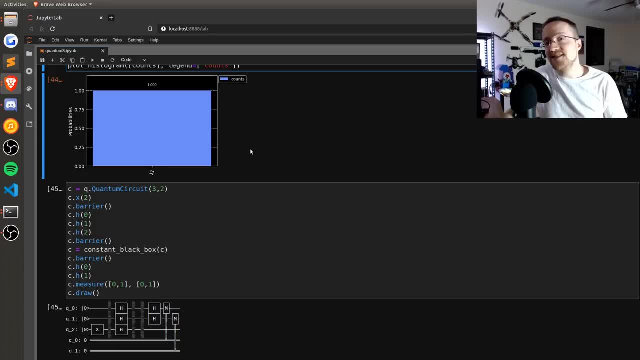 this circuit and output that instead. So then, so then, what we can do is: clearly, there's more information here, right? It's not just a simple zero and one. There's so much more to the story and we can work with that intra circuit. That's what that's: the, the, the. 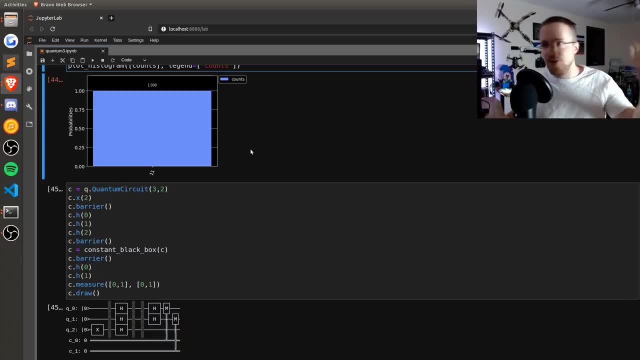 the real amazing part of all of this. It's not: oh, we did it in one shot. It's. why did we do it in one shot? So, uh, with that we're almost done here. The, the, the last thing I want to show you. 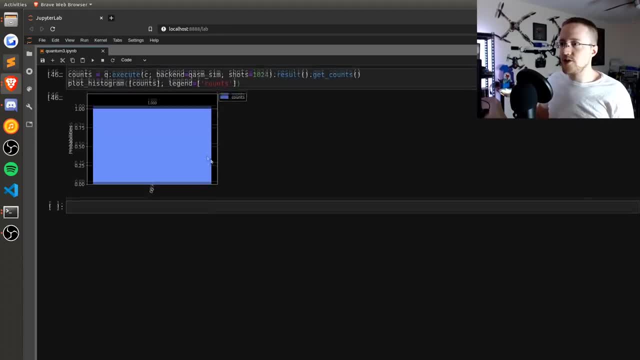 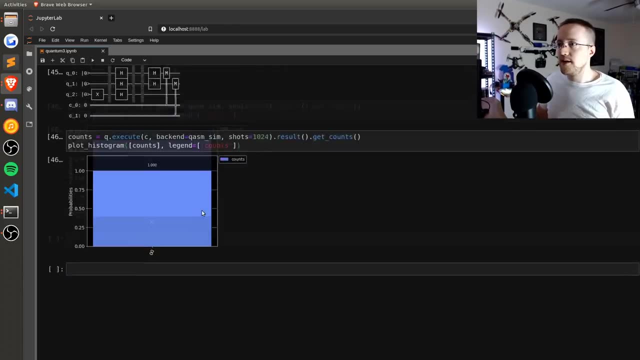 is what I asked earlier, which was: can we? I don't know if I saved it up here. I was hoping to just copy paste, but I don't think I did. Can we mimic? um, let me just take a circuit real quick. 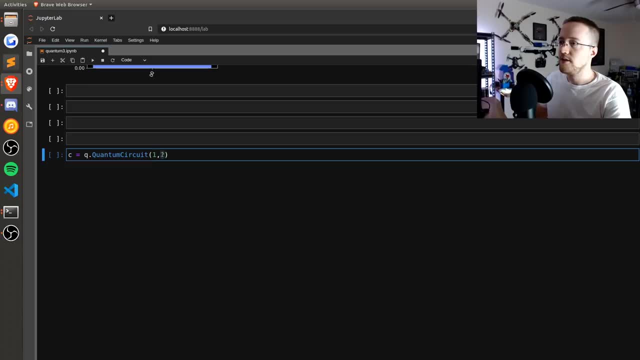 Can we mimic? uh, we'll do. uh, one one, Um, the Deutsche stuff is basically over. Um, well, I guess it's not, cause I'm going to make a point, Um, but anyway, now we're just kind of screwing around again. 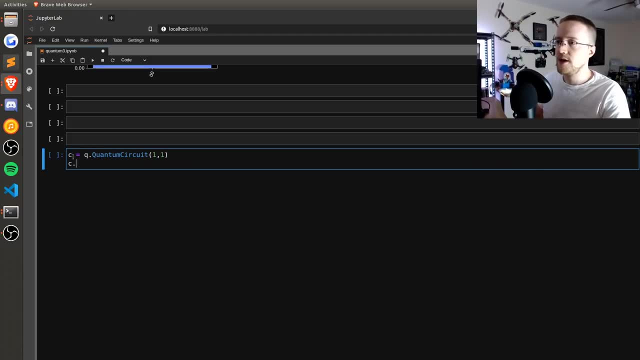 You don't have to follow along, You can just watch. Um, so we have a quantum circuit, We have a CX zero. Uh, so a, not a Hadamard on zero, Uh, we don't really have to draw, but I'll just do it. 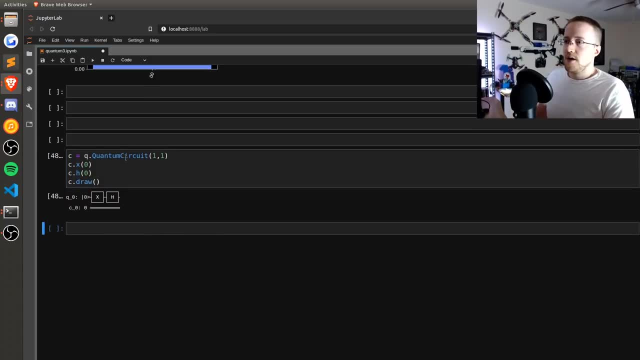 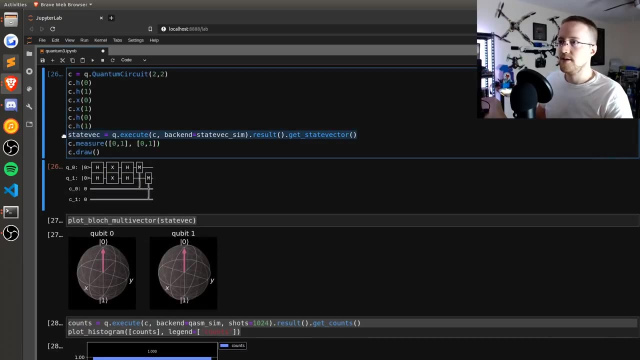 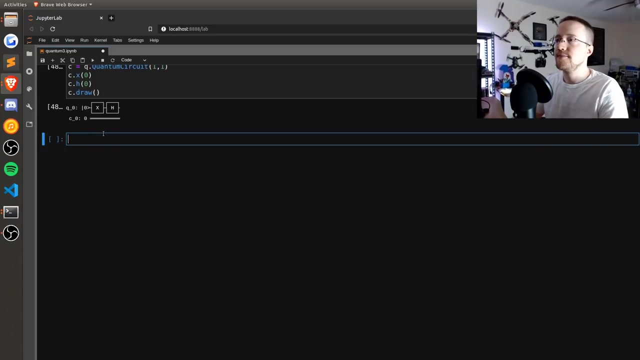 Uh, C dot draw Um. and then we want to state vector. Where is a state vector code? You know what I'd really like? You know it'd be awesome: Kiss kit devs like C dot draw multi-vector. That's what I want in my. 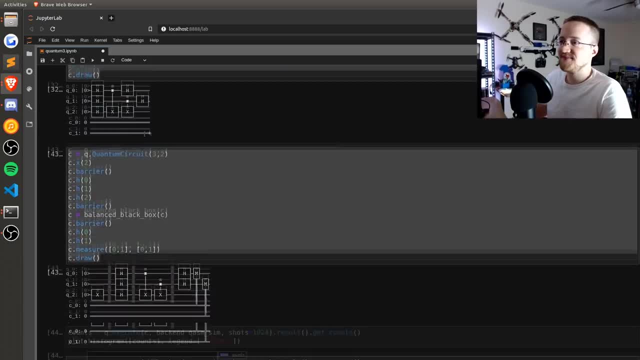 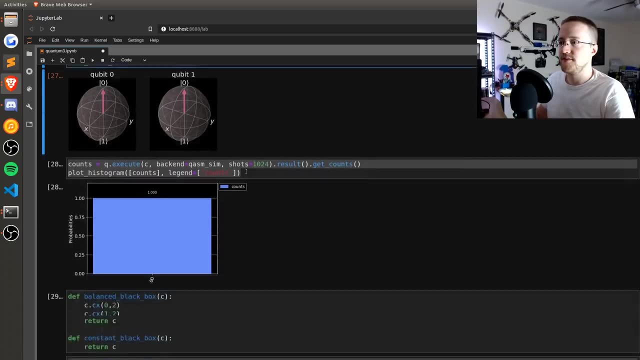 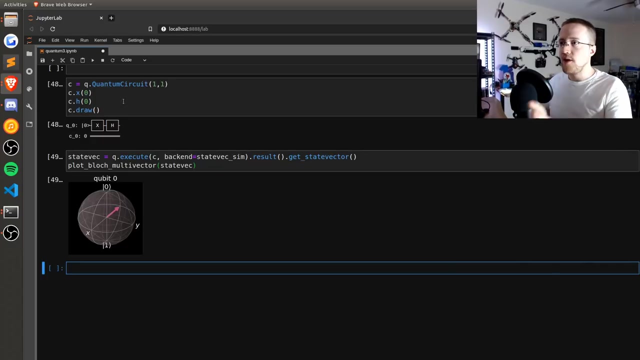 life. Um, cause, like doing this every time you want to make the drawing. Uh, multi-vector state. Okay, So that was that way. And then if we were to flip the Hadamard and the knot? so what if we did Hadamard, then a knot, Cause don't forget as well. Um, if we just have? 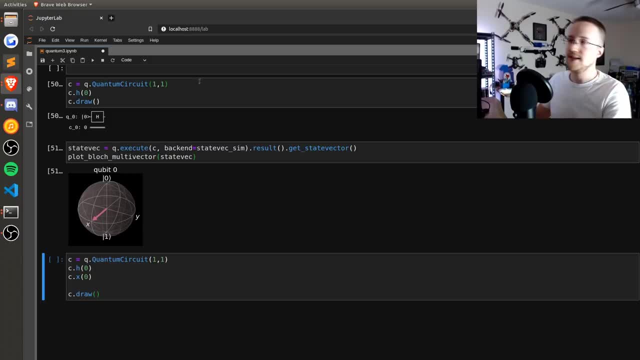 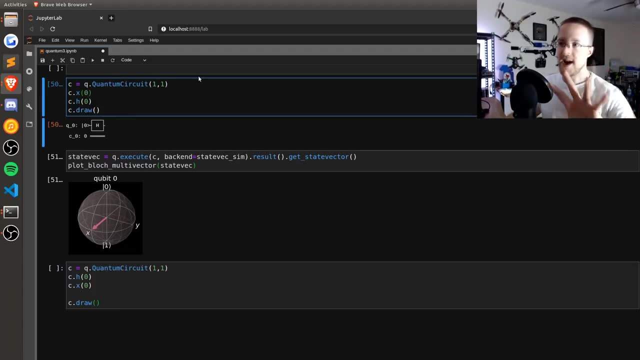 a Hadamard, what? what did that look like? Right, It's fully in the X, And then if we have CX, Hadamard. so this is the order of a knot Hadamard That we have in our um. do? it shows the algorithm. We can see. oh okay, It flips it around. 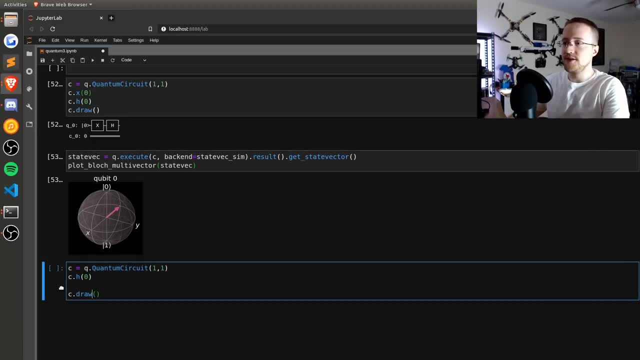 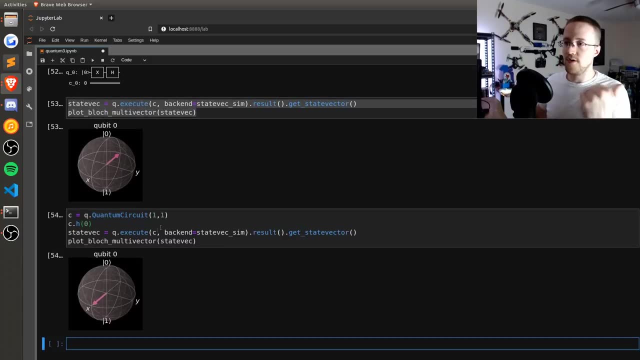 Right. So again, if we do- and I'm going to stop drawing X, that way we can do all this in one run- I'm just going to say boop, boop. So again, Hadamard, all the way. And then if we, if we put, 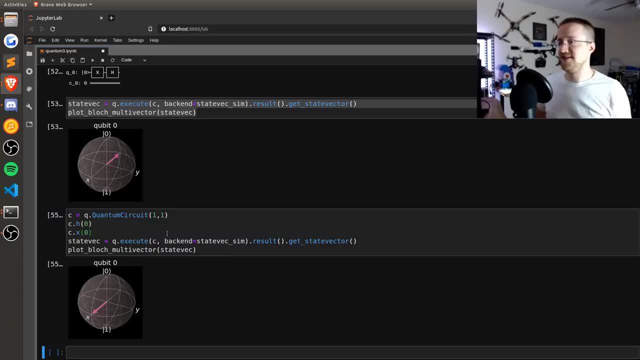 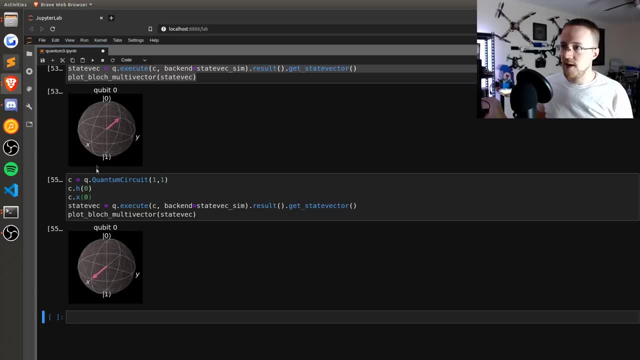 00, 00, 00, 00, 00.. When we go from X to this like negative X: Um, what's going on? How, how else could we get there? Could we get there some other way? Um, so, like from here could. 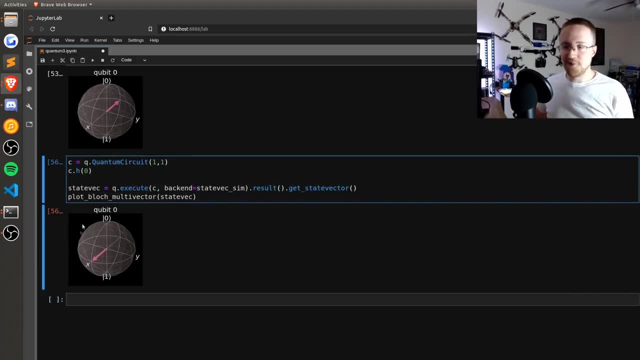 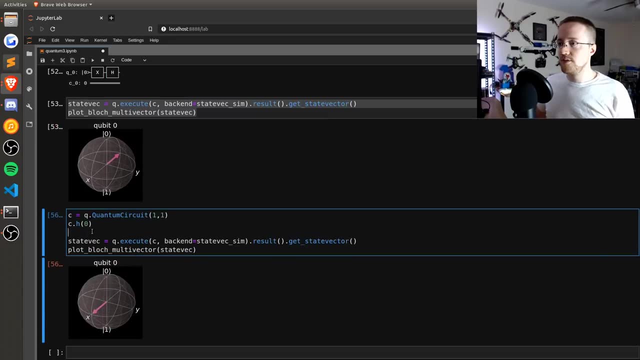 we get there. Of course we can get there. Remember, all the gates are superposition, entanglement in a rotation. So what if we say circuit dot rotate on the Y and we're going to rotate by math dot pi on qubit zero. can we get there? it turns out we can. we can get there. 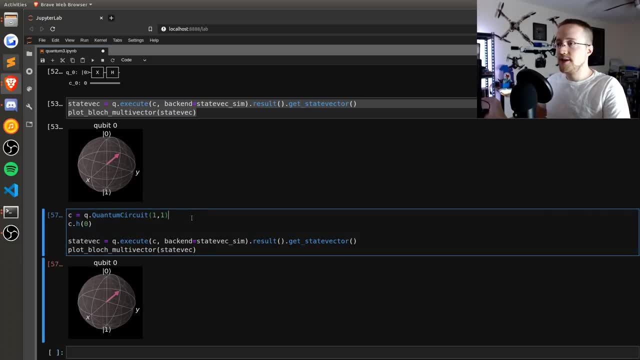 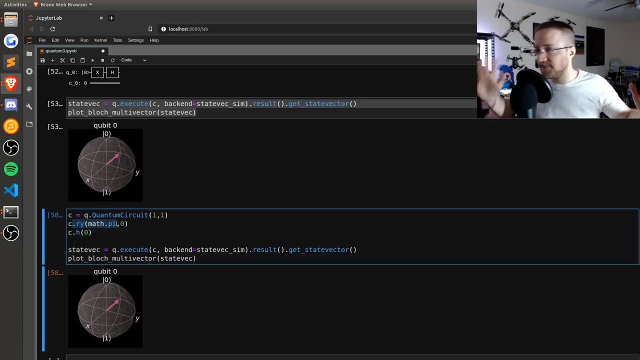 after the hadamard. we could also get there before the hadamard, so we could. we can throw this rotation on the y anywhere the heck we want. the next question is: does this collapse in the same way as we would hope and expect? now, i could, we could do it with just the circuit, but instead 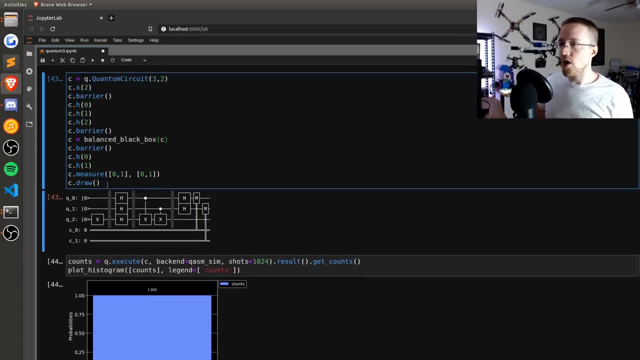 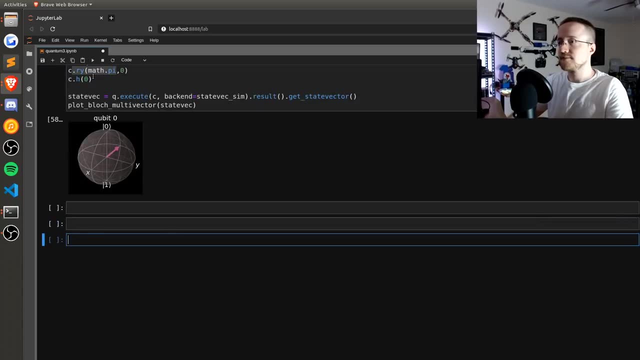 what i'm going to do is: let's take what everything we've been doing up to this point. so we're going to take this now in theory, right, this not this is what we're trying to wonder. hey, could we change this? so this not, as you've. 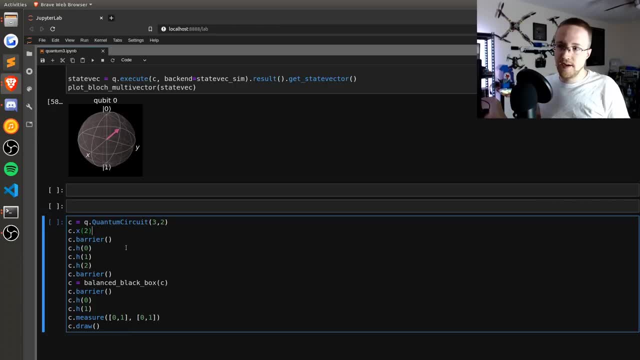 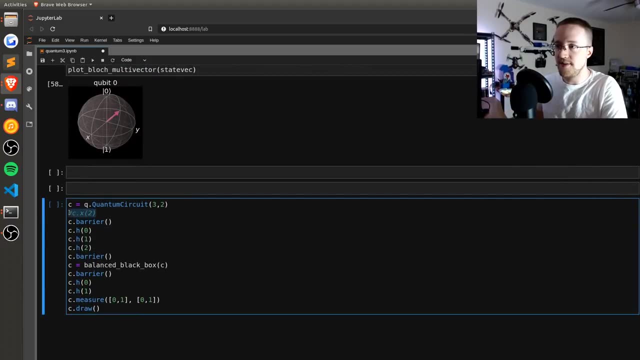 already seen, if we put it after the hadamard, it doesn't work, at least in our simple example. now i can prove to you. it also isn't going to work here. so, for example, i'm going to comment that out and then we're going to move it um here. so we'll move it after the hadamard and then we'll do. 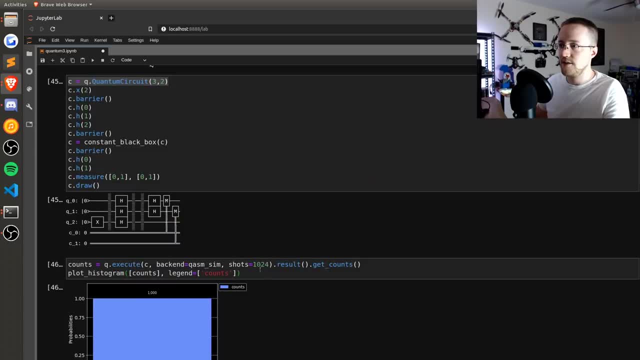 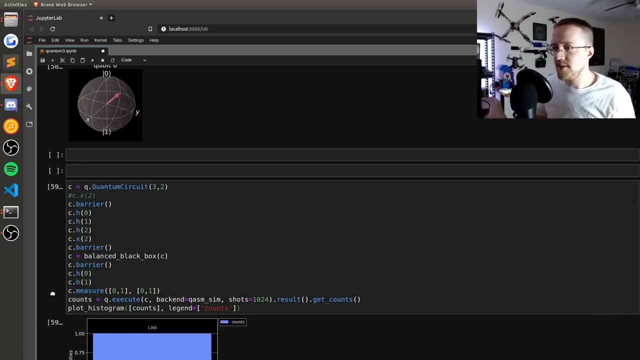 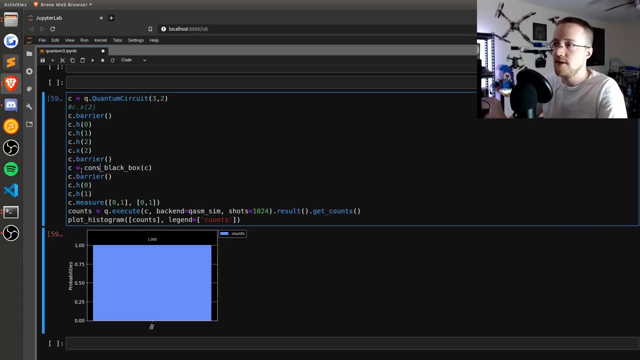 um, let's just take uh counts here copy come down here. um, i don't think we need to draw it, so again, i'm just going to run everything immediately. so we get a zero, zero on the balance box. and then you might be thinking, well, maybe the constant is a one, one constant black box. it's not, we get zero. 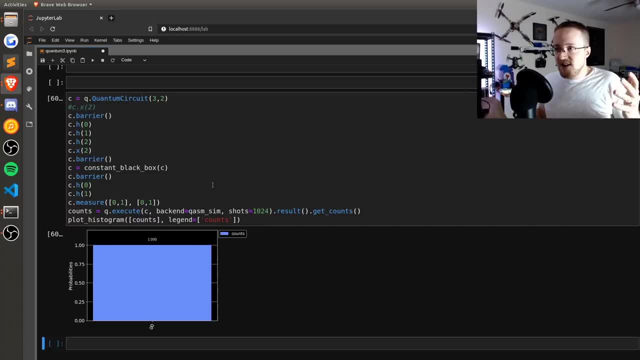 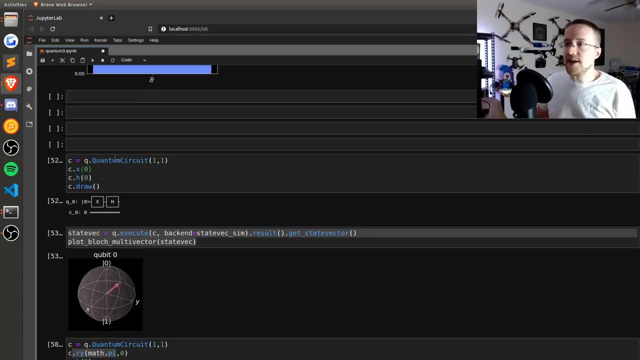 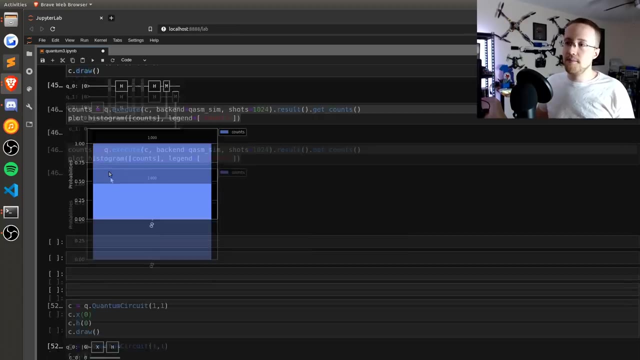 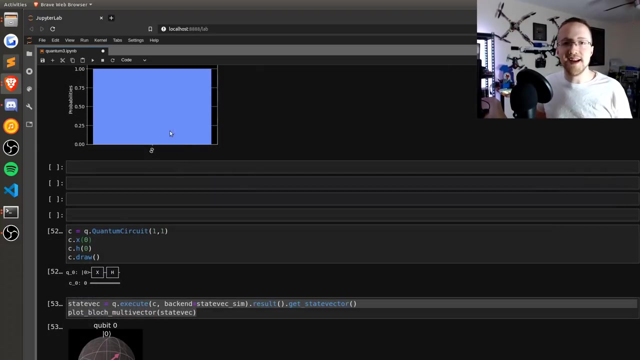 zero across the board. so we've lost our um, the attribute that was so cool. and we, we can understand. maybe not the, the quantum mechanics in the background. maybe we don't understand that, but because we, when we actually graphed the- uh, the multi-vector- i don't know where my option, my example, went, but when we did, you saw it didn't do anything right. 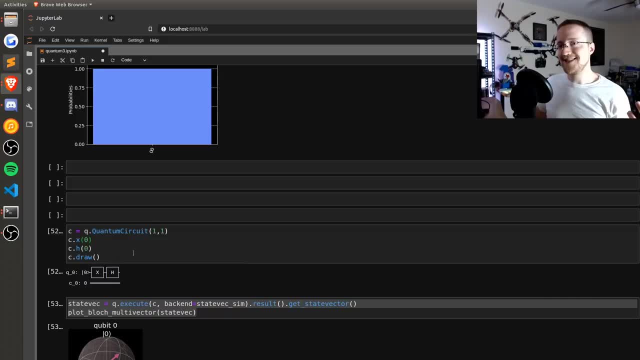 you hadamard, it was full x. you did a not, it was still full x. so it's no surprise this is not working, but we're going to do it again, and we're going to do it again, and we're going to do it again, but what about? 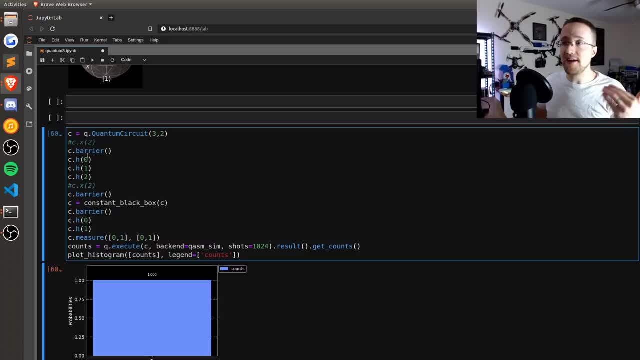 i'm going to comment that out again. we're going to say a rotation now. so we're going to. we're going to replace the original formulation, where there's a not before the hadamard, with a rotation on the y instead. so we're going to say math dot pi uh, qubit number two or index two, rather run it. 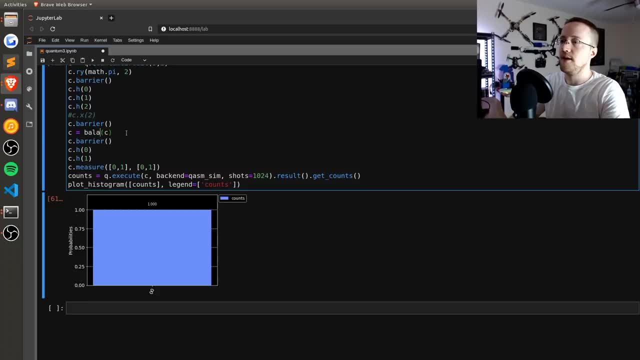 okay, constant is a zero zero. uh, i don't want to rewrite the whole thing. probably could have done it by now, though balanced black box, and then we're going to do it again. and we're going to do it again. like we said, we're going to go back to the original formulation, where the rotation on the capture 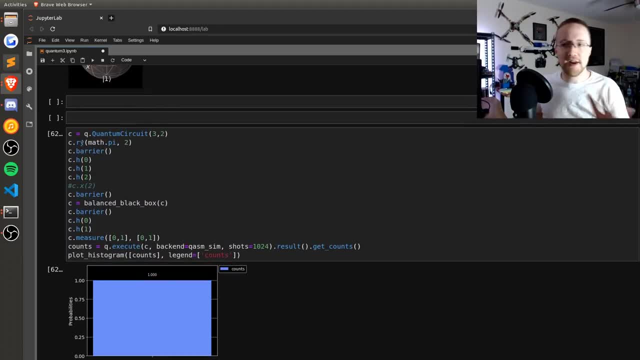 the distance is, what we're going get is one-one. so now we're going back to the again here. we're going to make the same adjustment again. so we begin here. so we start with a inevitable. but, as we've also seen, we can get that exact same behavior right, and as long as we're getting. 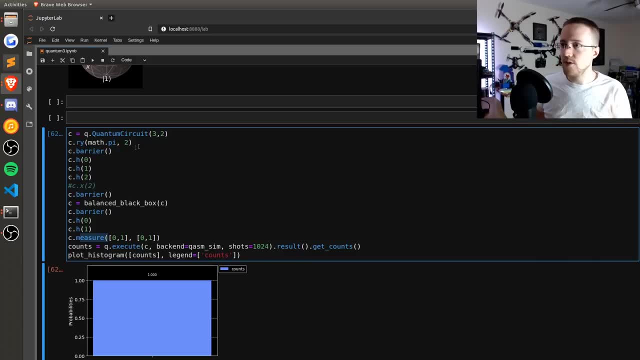 it before we take this measurement. we should be fine, right. so the question is: okay, can we take this rotational y, remove it from there and'd apply it here where the controlled x or a control, not rather um or not, not a control, not the not gate did not work. So we run this on the balance. 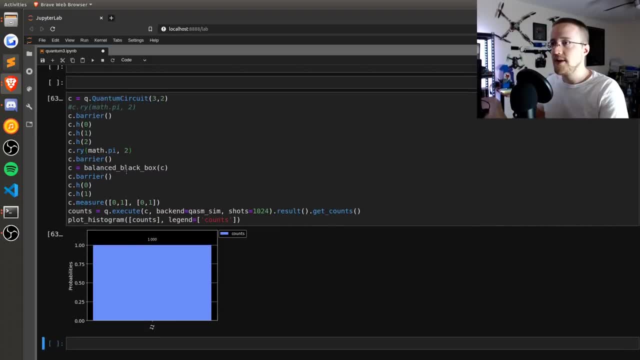 box, We get a one one again. Good, That's what we hoped. Now can we do the same thing and get it on the constant black box and get it, Hopefully, a zero, zero. we can, So I'm going to leave it. 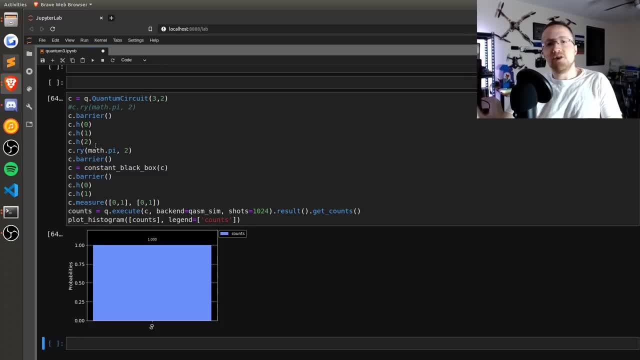 here and just leave you with this. that again, you, you don't. the math might allude you as to, and it alludes me, why the not didn't flip the Hadamard back the other way, Right, Um, but then 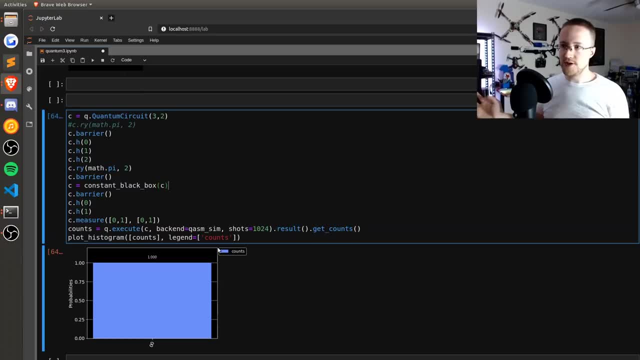 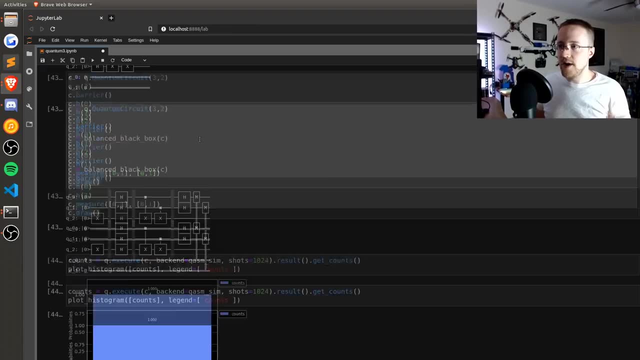 like I said, as I'm just kind of playing with this Deutsch-Josa algorithm, I'm like, Hmm, that's interesting. You know, cause, in theory, you, you just need to make sure everything is the same: either have a balanced or a. constant balance box And then you just need to make sure everything is the same. either have a balanced or a constant balance box And then you just need to make sure everything is the same. either have a balanced or a constant. you know thing that happens at this. 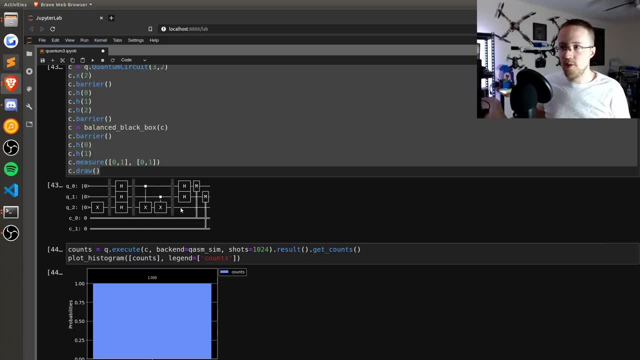 point. So as long as we do our operation before we get to the C knot, in theory, uh, we should be fine. And then, as long as nothing else changes here before the measurements, again, you should be fine. Or as long as before the measurements. you either have a constant or a balance. So 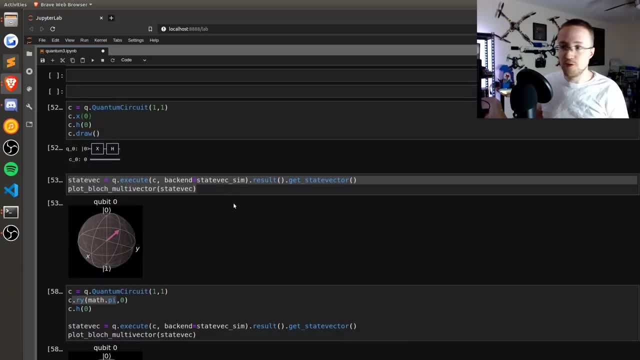 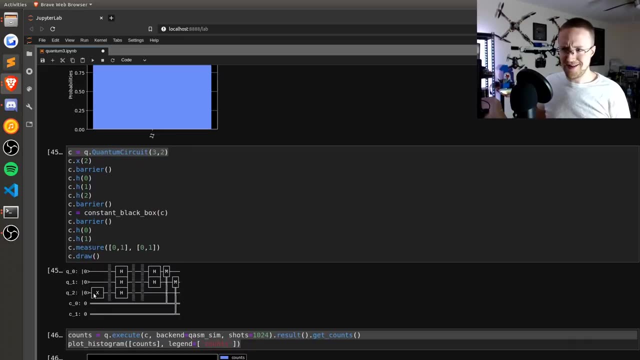 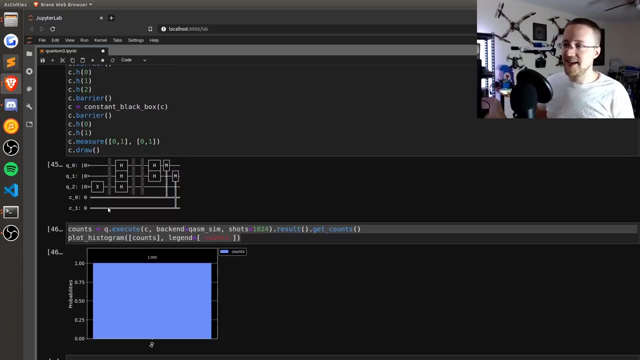 anyway, I was playing with it and I was like, well, is there another way that we could get this? Like I was curious: do we actually have to have this, not gate here? Like why can't it be here? And then I plotted the multivector and I was like, oh, it just can't be there. And then I was like 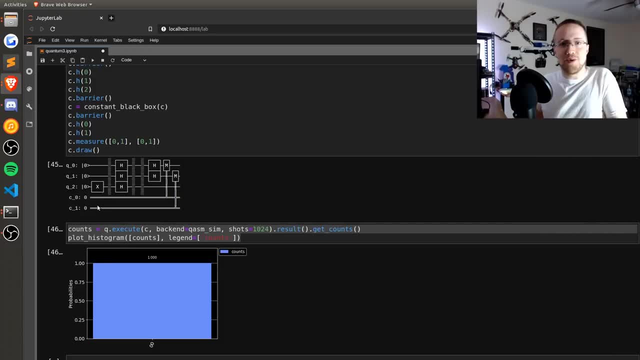 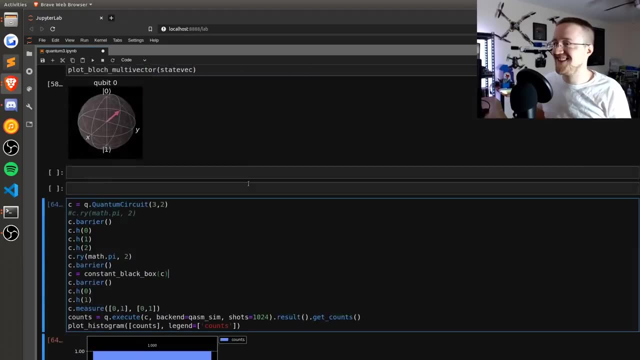 but that's weird. Why doesn't it move the multivector? And I'm like, well, what if we do a rotation, Like surely that will move it Right? Um, and it does, and it works, at least on the sim. 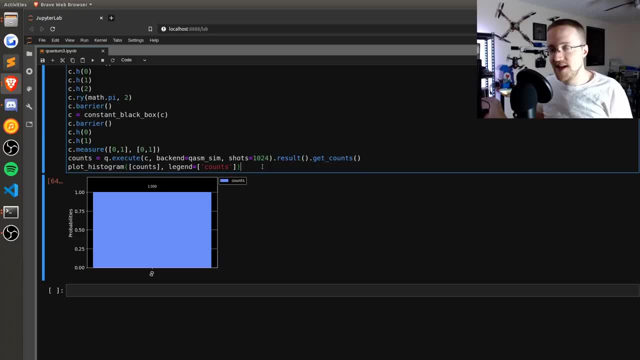 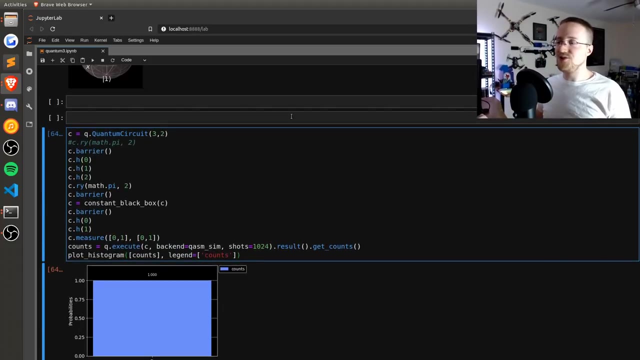 So, anyway, very interesting. So that's it for now. If you know the proper terminology for a multivector, uh, if I've said anything else stupid, feel free to let me know. Uh, but yeah, that's so cool. Um, so hopefully you guys are as intrigued by all this quantum uh computer. 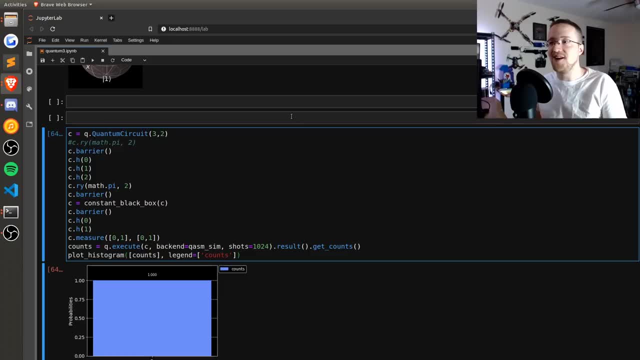 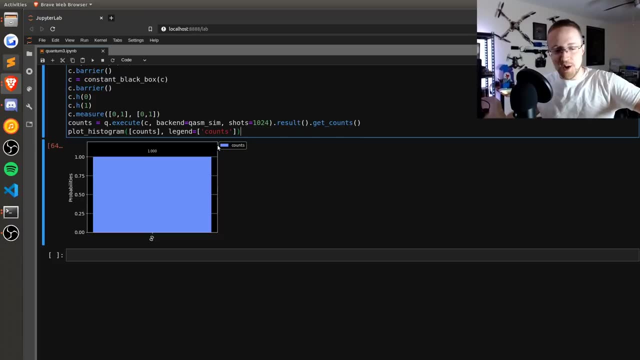 programming as I am, I'm having a really really good time playing around with all this stuff. This is just super interesting And it's really cool to see all. it's like the, the it's just a complete, it's just totally different. You have all these possibilities and like what we're going. 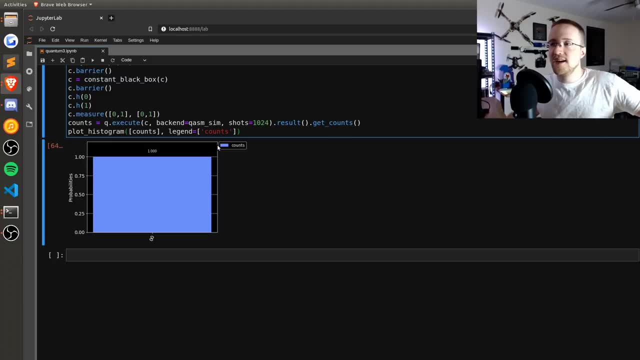 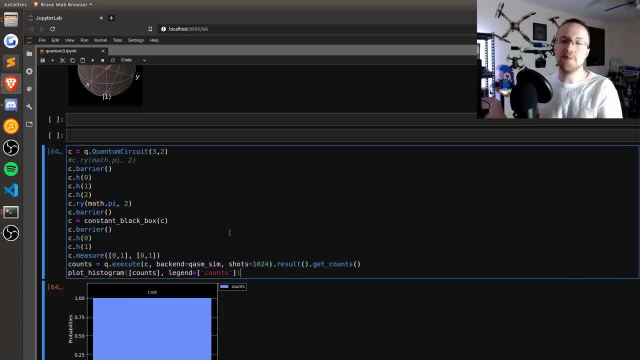 to be able to do with. that is very interesting to me, Um, as we move forward. So, again, while this might not be an, as an algorithm, all that interesting, it's very simple, So it's easy to understand. but this concept, this is the inspiration behind Bernstein. 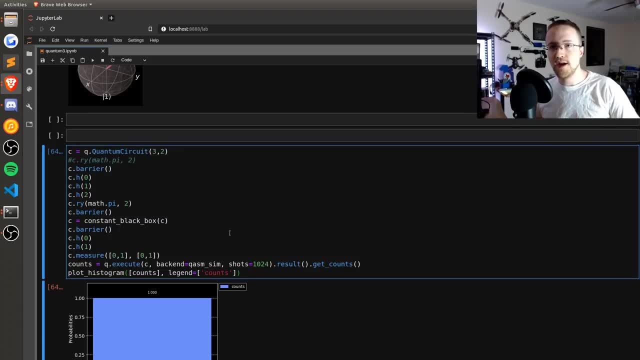 Boz Rani, which is basically a way that you can encode um, a bit string, into your circuit Um. and then there's the shores algorithm, which is the one that you know can factor large prime numbers. So factor four large prime numbers, So anyway, and in effect, break, break and. 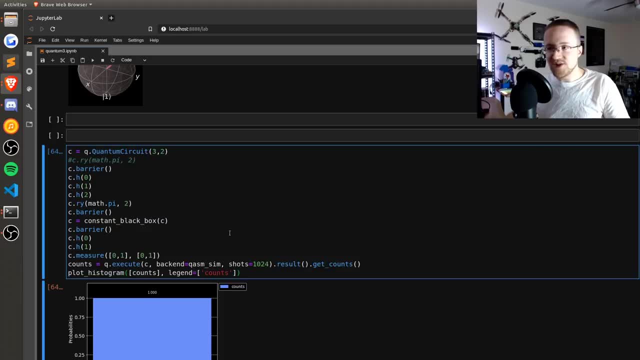 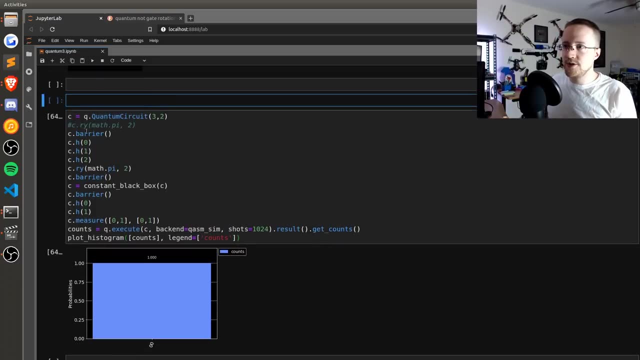 correct. So, okay, I think that's all. So you thought you were rid of me, but actually I wanted to stress one, one final thing, Uh, and that's in relation to why did the not not work? And then, 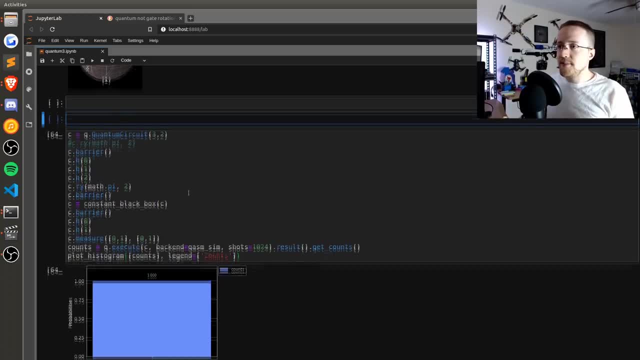 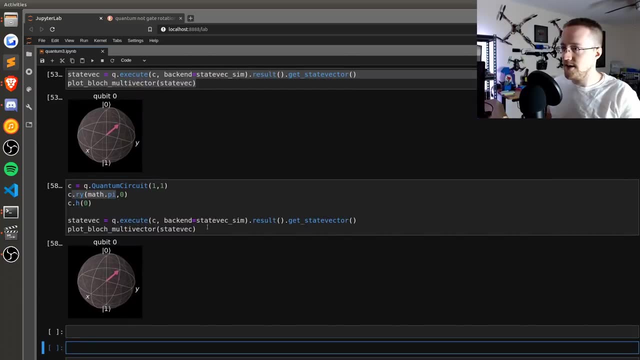 the rotation on the Y did work. Um, I don't think I didn't make that totally clear, Like it might be like, Oh, why did that happen? Um, there's a reason, it happens, So, uh, so what, I'm going to. 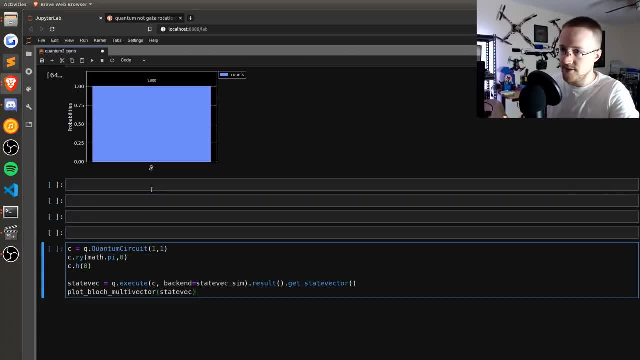 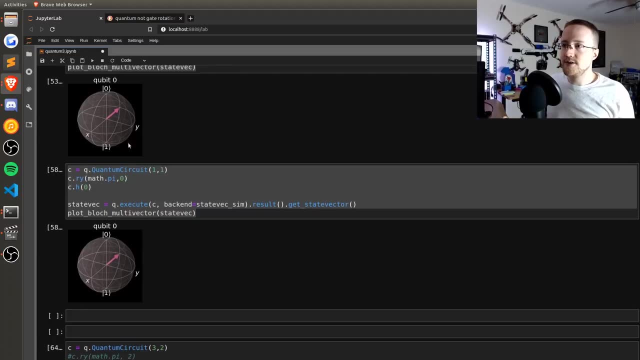 do is I'm just going to take this here and real quickly answer that question. So what is the rotation or what's a not gate, right? So so with our Hadamard? uh, we've lost it. Okay, I'll. 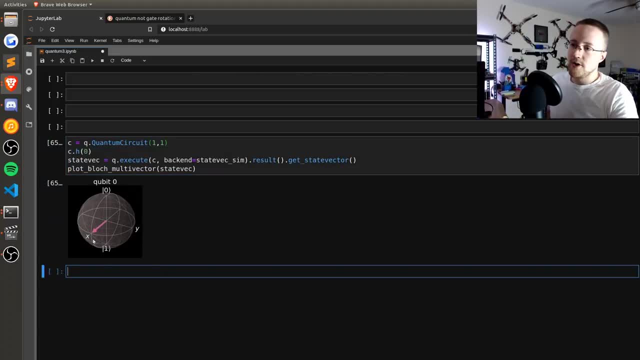 just do it down here. Um, so our Hadamard goes to here, or, even better yet, let's say, let's do, let's just do nothing, And then we'll add a not gate. So so this is our start. We initialize to: 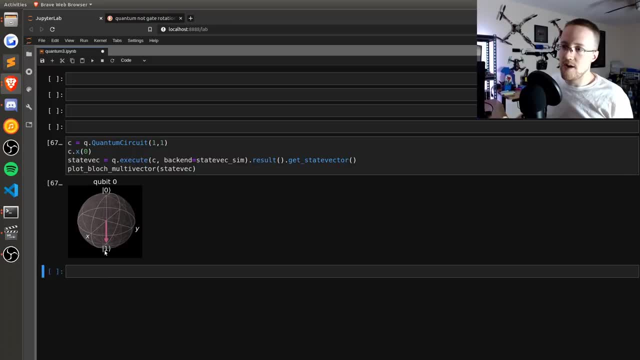 zero. Let's say we apply a not gate. Now it points to down to one. The question, though, is how do we get to one Right there? There's two ways. we could have applied a rotation to cubit zero to make our way. 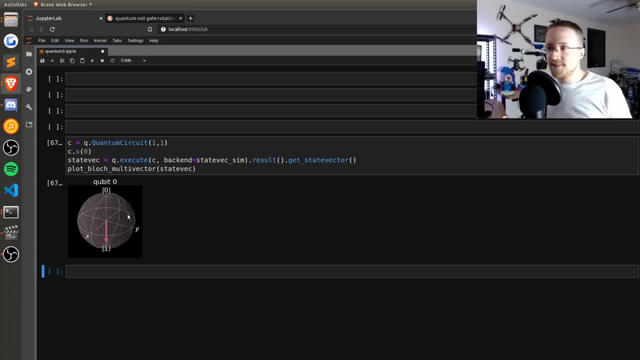 to one. One of the ways is to rotate along the. let's say, one of the ways was we could have rotated along the Y axes to get to one. The other way is we could have rotated along the X axes to get to one. The dot X should give you an idea of what happened. right, But what if we said: 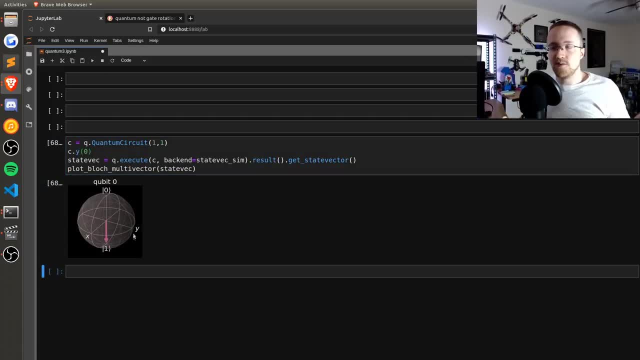 what if we say C dot, Y, zero? we get the same result. And you might think, oh, I didn't even know those existed Right. And you also have a control Z right, Cause here's your Z axis, right here. So, and and when we do a CZ on what otherwise is already pointing, you know if